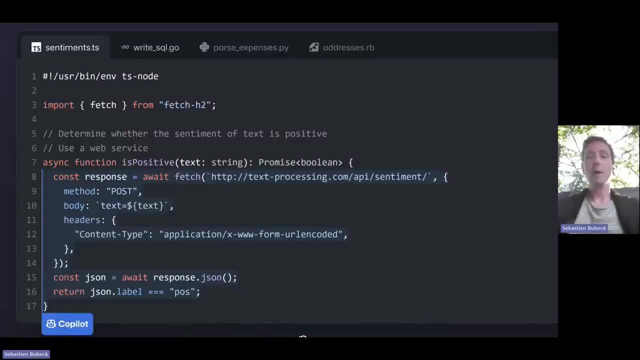 What are we talking about with large language models for coding? Well, we're talking about things like copilot, where you give the beginning of some code and then you ask for basically a completion of the code. 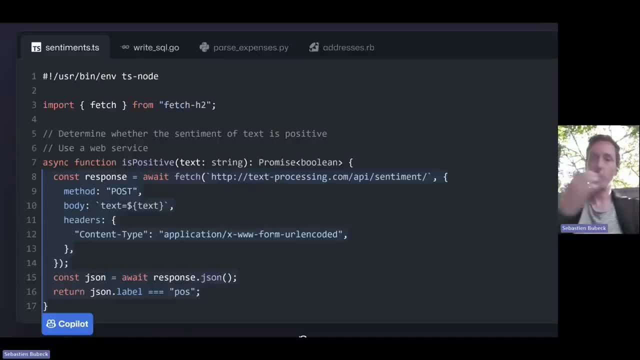 This is what those large language models for code are doing. OK, so we're going to tell you a new models like this with only 1.3 billion parameters. 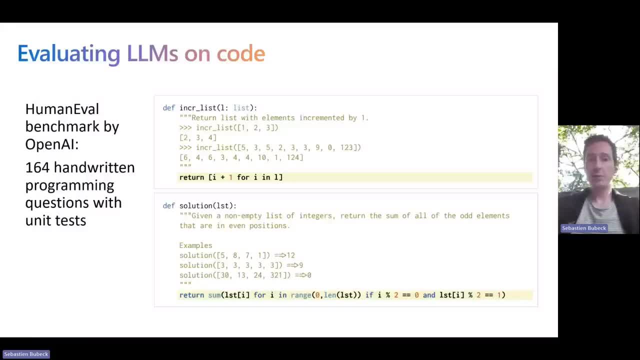 That does this kind of code completion. Now, the question, natural question is, how do you evaluate the performance of an LLM on code? And there is a quite standard benchmark by now from OpenAI called human eval. 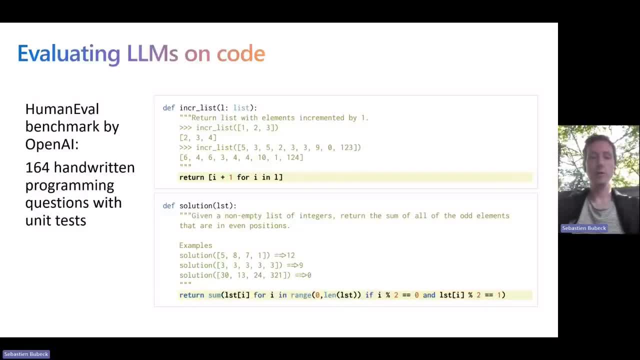 So this is one way to evaluate coding models. This is 164 handwritten programming questions with unit tests. So each of those programming questions comes with a set of unit tests. And you say that, you know, you have solved the task if you can pass all of these unit tests. What do those programming questions do? What do those functions look like? They look like this. You get the name for the definition of the function, like increase list. And then you get a doc string explaining to you what, in natural language, what the function is supposed to do with maybe some example. 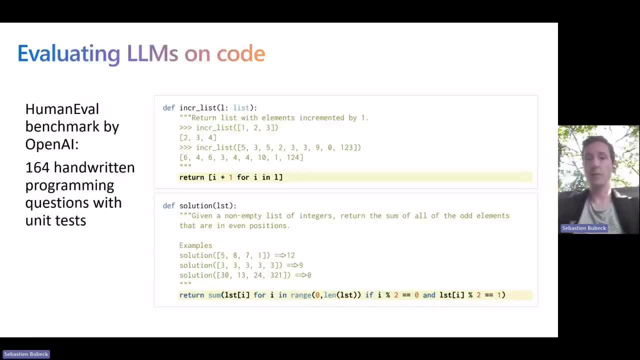 And now the goal is to complete, you know, to write the code that does what the doc string is asking you to do. OK, so here, just two examples, one where you have to return code that, you know, given a list, increase all elements by one. 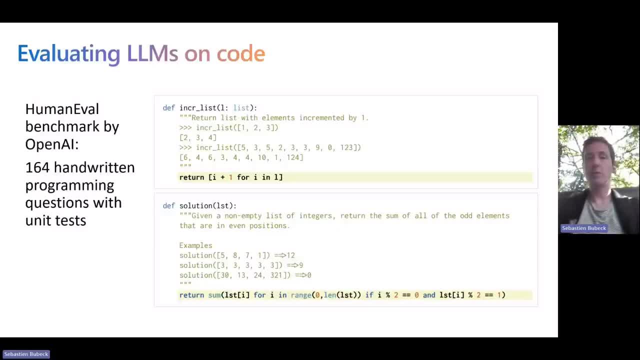 And this other one is given a list of integer, return the sum of all the odd elements that are in the event position. So you see these code completions are very easy. It's just one line of code. So this is very simple. 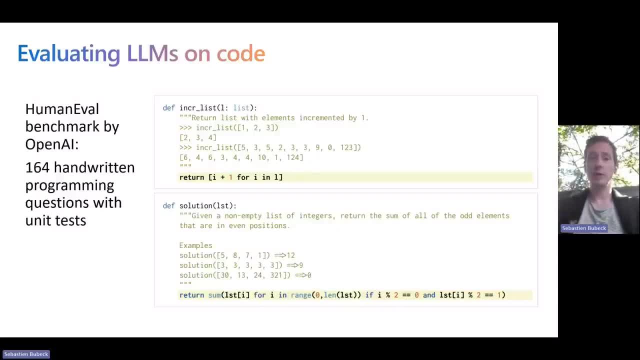 But in the human eval benchmark, there are also much more difficult coding questions. Now, let's look at the progress that have been made on this benchmark in the last couple of years. You know, as you all know, AI has made incredible progress recently. 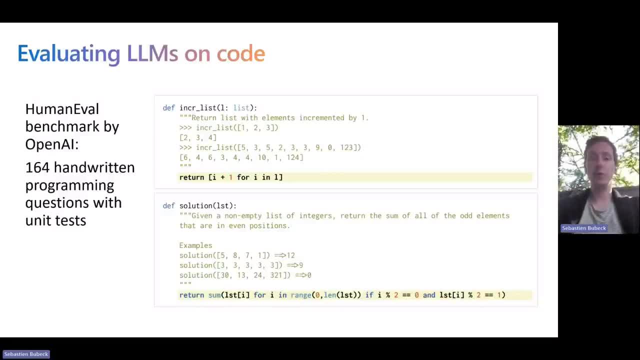 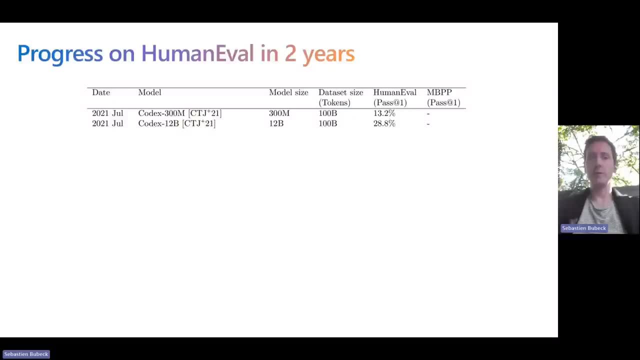 Let's see how it looks like in action on this specific benchmark. Let's see how it looks like in action on this specific task of coding and specifically human eval. So human eval was introduced again two years ago in July 2021 by OpenAI. And at the time, they created also two models, you know, the Codex series of models. And these were coding large language models. And here I'm giving you two examples. One is a 300 million model and one is a 12 billion parameters model. So you see here is the model size. Both of those models were trained on 100 billion tokens. Okay. So this is the size of the data set. 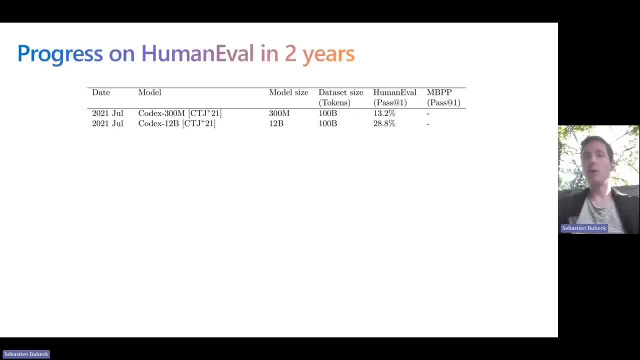 And what scores did they reach on human eval? Well, the 300 million only got a mere 13%. 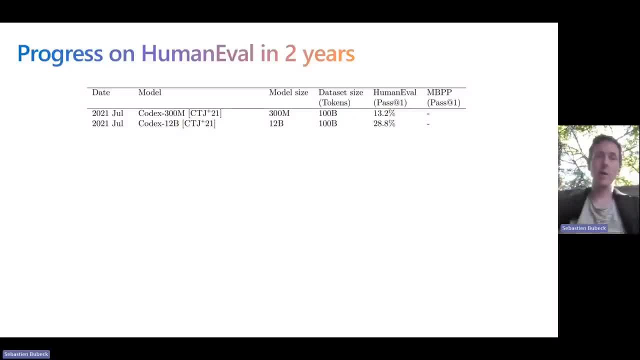 While as you scale up the size of the model, you get this amazing, you know, fantastic magical behavior that as you scale up the model, the performance improved. And you can see a huge jump to almost 29%. Okay. So this was two years ago. 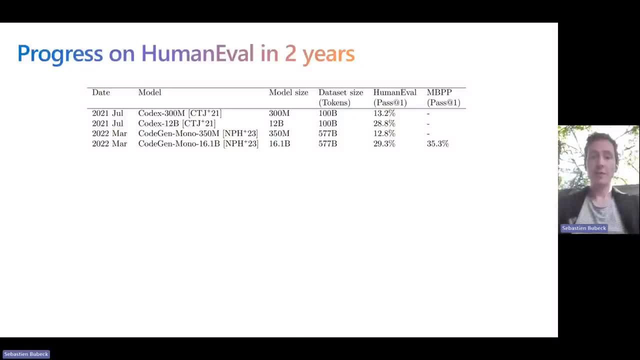 So what happened since then? Well, shortly after, something interesting happened. 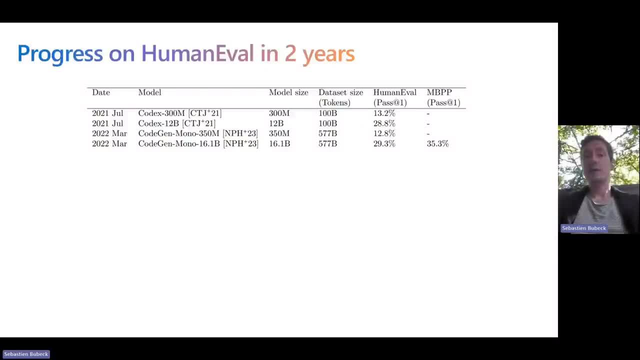 These folks at CodeGen, they created a model trying to mimic OpenAI, but they open sourced their model. They obtained very similar results. 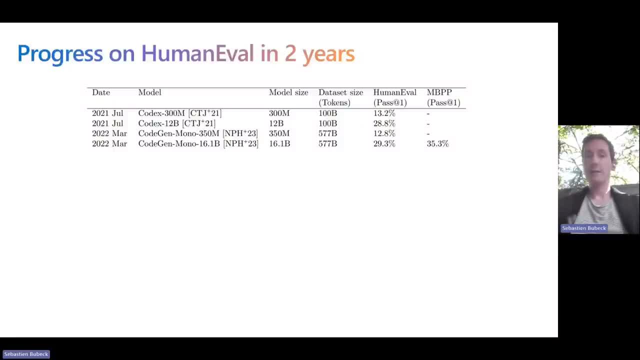 You see that at 350 billion, they also got 13%. At 16 billion, they got 29%. They had a data set much bigger, 500 billion tokens. 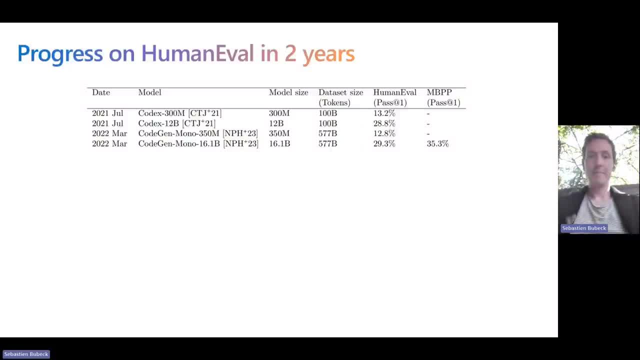 Yet, you know, no real improvement in terms of the human eval. Now, after that, things started to heat up a little bit. 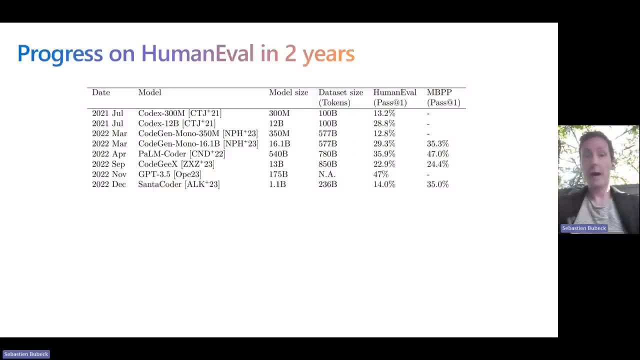 And you can see the big model. It started to emerge with Palm Coder, specifically, 500 billion parameters, a much bigger data set. 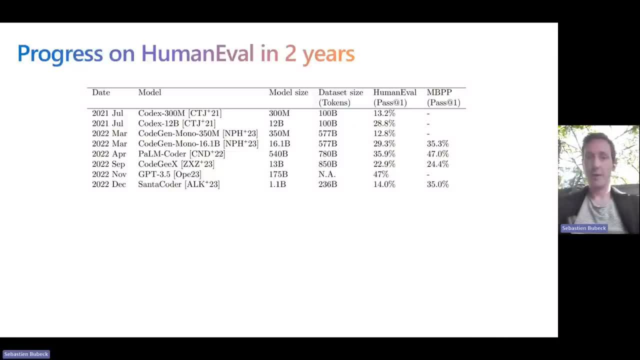 You know, we are now nearing the 1 trillion token, 780. And you get, again, a little boost. But you see some kind of diminishing return. You know, we moved from 300 million to 12 billion. We got a 2x improvement from 13% to 29%. Now you move to 12 billion to 500 billion. And you only get an improvement to 35%. 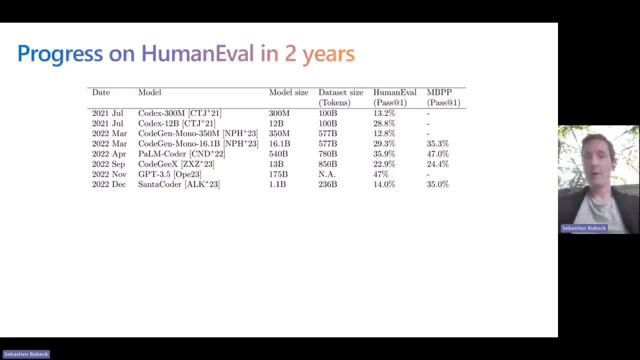 A little diminishing return. Of course, GPT-3.5, we don't know the size of the data set. 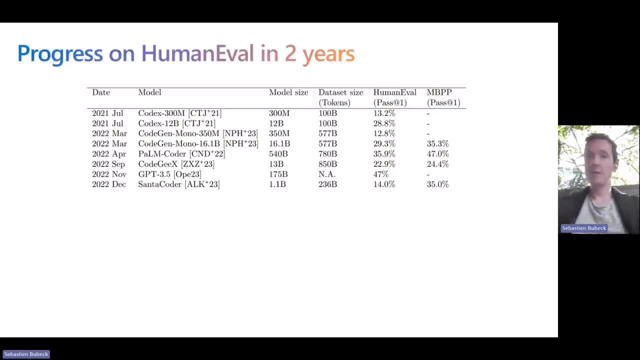 But this is 175 billion parameters. And this reaches an amazing 47%. 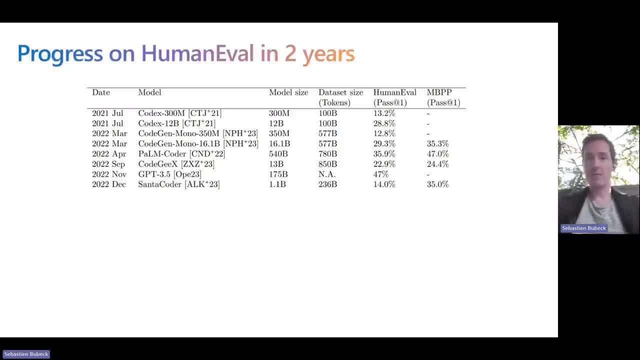 Other models, you see, they are increasing the size of the data. And you get very little improvement. 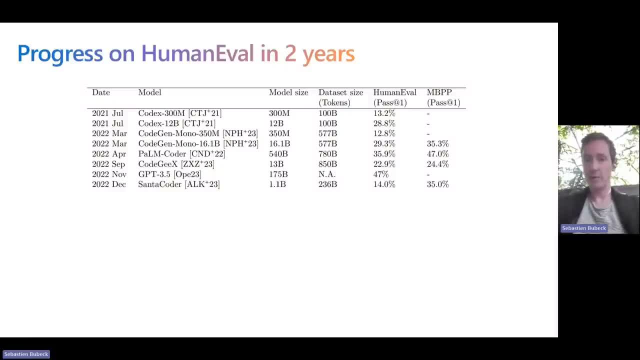 Here's the Centacoder. It's interesting because it's 1 billion parameters, like the model that I will tell you about. 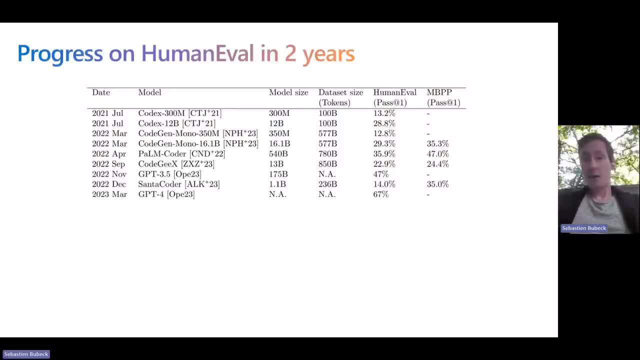 And it reaches only 14%. But then, of course, GPT-4 happened roughly six months ago. 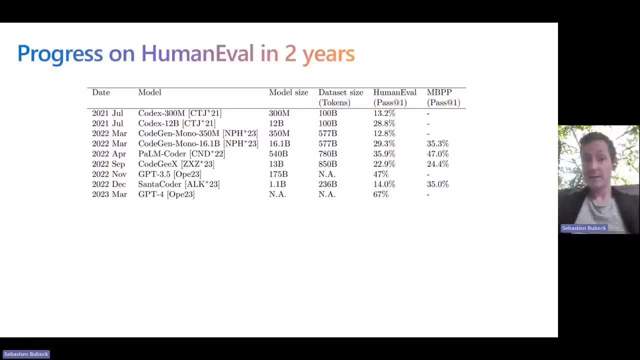 And this made an amazing jump to 67% on HumanEval. 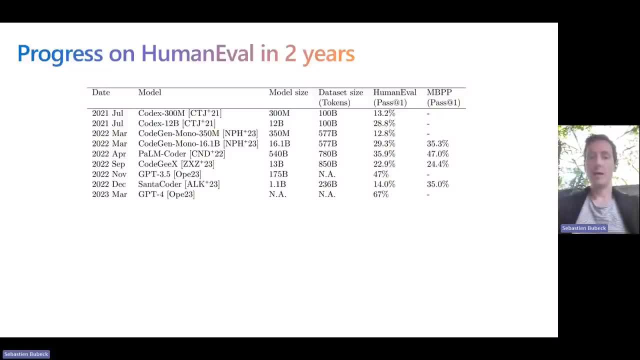 And, in fact, this is a version that was released in March. But the version we had access to in Sparks even got a higher score. 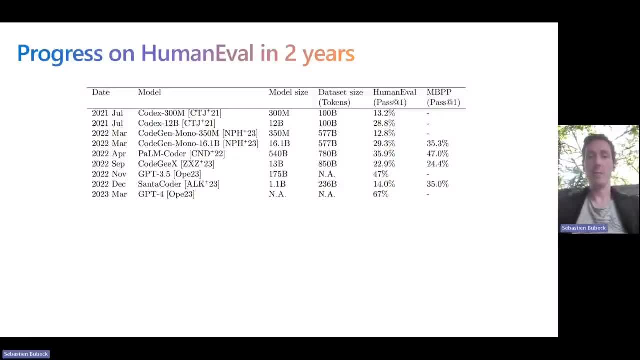 So GPT-4 really kind of cracks the problem. Now, shortly after GPT-4, things really started to heat up. 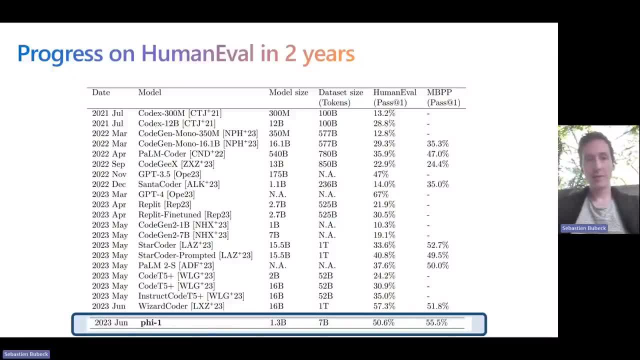 And we see that we have new models coming out every month. In fact, in May, we have, like, many models that came out. And they all share rough parameters. And roughly the same characteristic. You see that the data sets, they are huge. 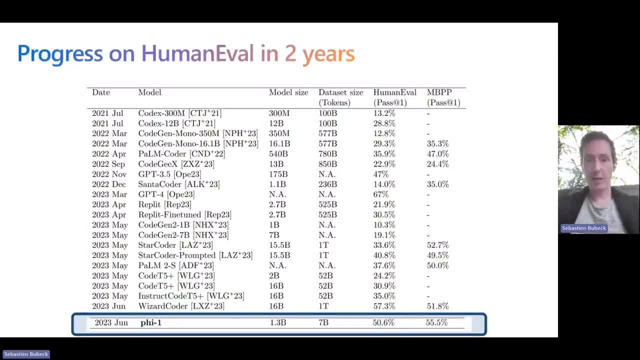 You know, 500 billion, 1 trillion. You know, some of the recent ones here are slightly smaller. 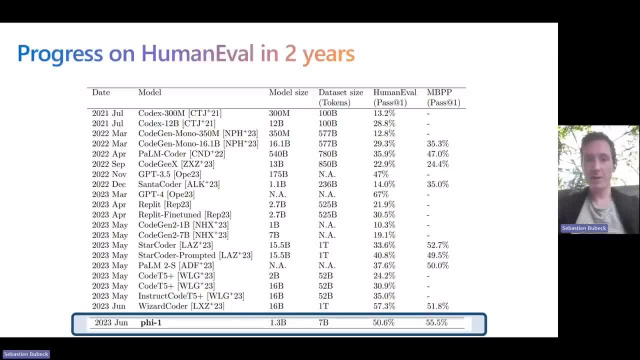 But the models are all big. 15 billion parameters you get in the 30%. 16 billion parameters you get, again, in the 30%, 35%. So you see it's all roughly in the same ballpark. Maybe with WizardCoder being the exception, which is a jump at 16 billion parameters. 1 trillion tokens. It gets to 57%. 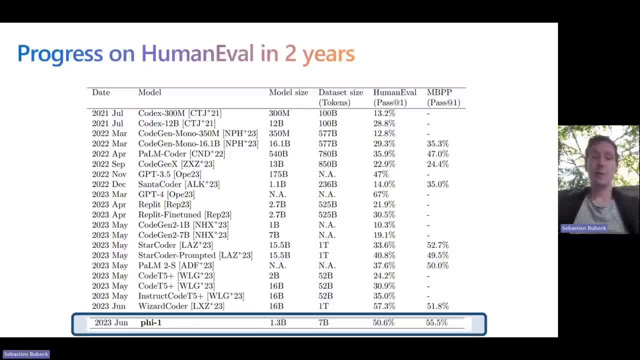 Now, let me tell you what we did. With PHY1 and the textbooks are all you need approach, which I will explain in a minute what it is. 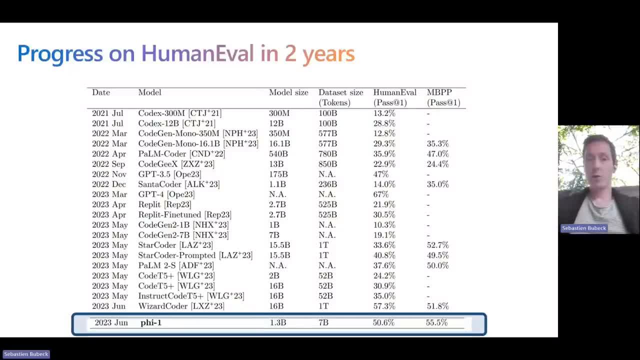 Here is the result that we got. We have a much smaller model. Only 1.3 billion parameters. A data set which is incomparable to those other data sets. Only 7 billion tokens. Yet we reach 50.6% accuracy. So except for GPT-4 and for WizardCoder, this is the best in this table. Despite being so much. Like three orders of magnitude smaller. 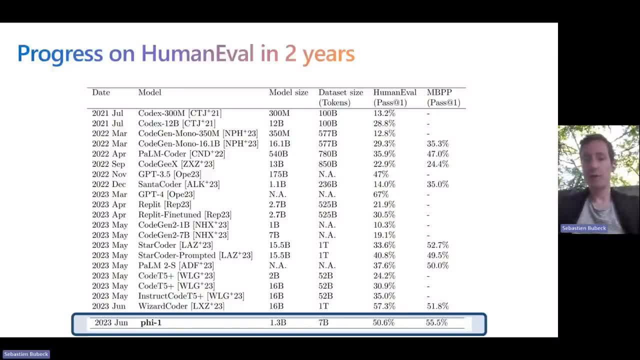 And moreover, you know, we're going to talk about whether we were overfitting to human eval. This is a very natural question. We will talk about it a little bit later. 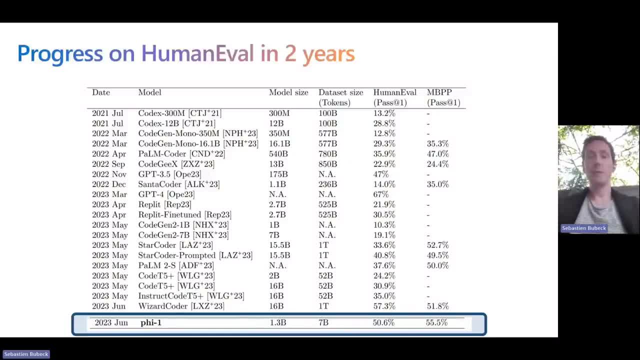 But I can already give you another benchmark. This MBPP, mostly basic Python programs or Python puzzles. We get 55% there, which is higher, for example, than WizardCoder. So this is just a small indication right now that we're not at least overfitting to human eval. 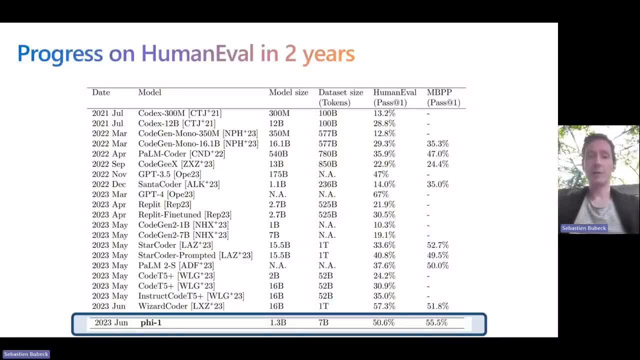 So now let me explain to you. What we did. What is this textbooks-are-all-you-need approach? 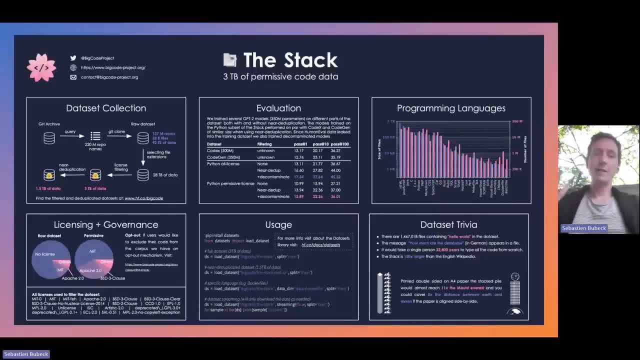 And for that, let me just backtrack one second. What are those data sets that all those models are using to train their large language models for code? 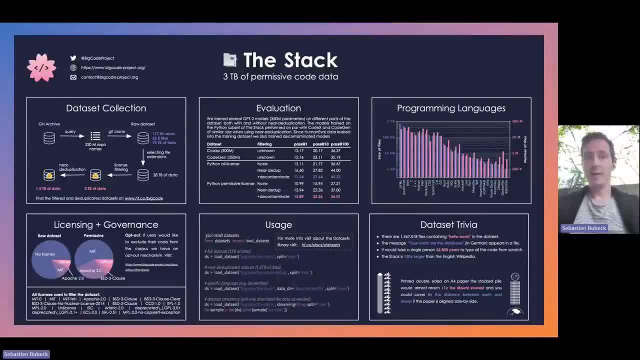 Well, one publicly available data set is this very nice data set called the stack. Which is three terabytes of data collected from GitHub. Which is under a permissive license. So we can use it to train. 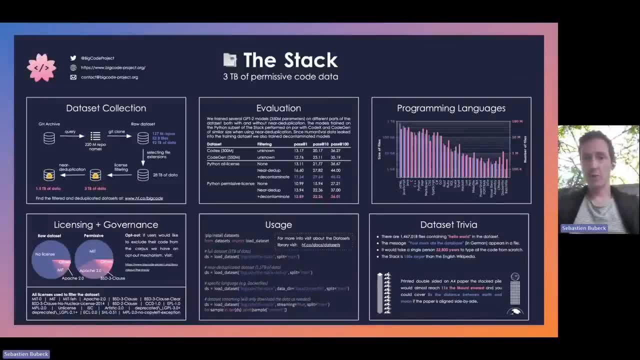 And these folks, they release the data set. And you can see here the distribution of programming languages. 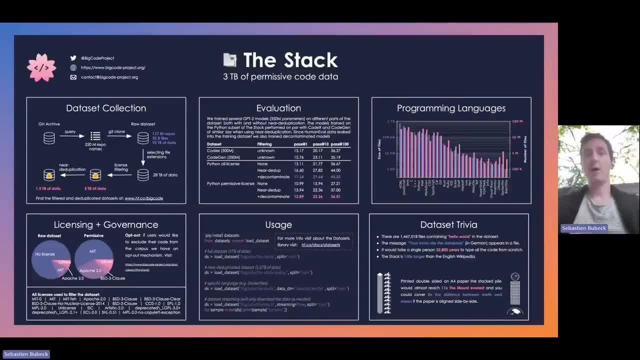 And we're going to look specifically at the Python subset of this data set. Which is made of 26 billion tokens. 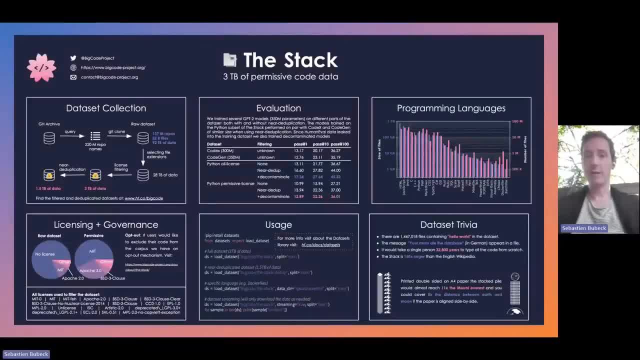 So it's a small part of the stack. And we're going to focus on that. Now, what does this data set look like? 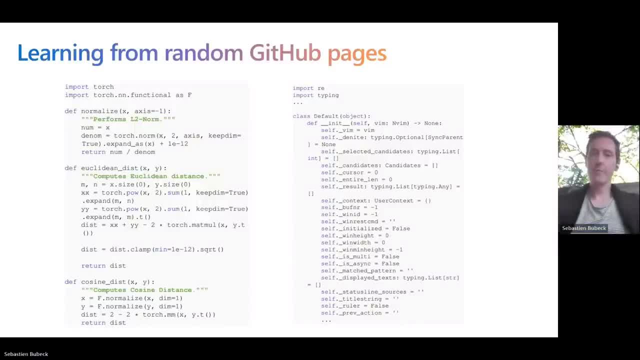 How does it look to learn how to code from the stack? Well, in this data set, you have documents that look like this one. 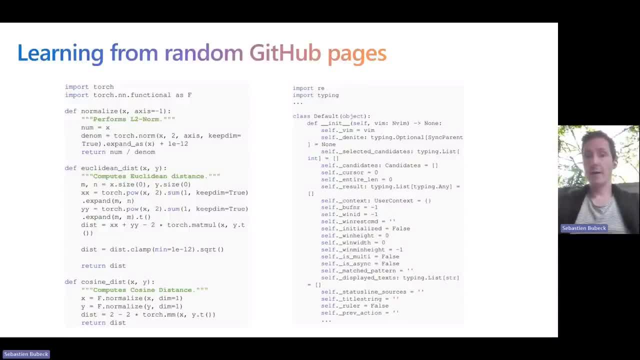 Okay. So, you know, you look at this code. Good luck to kind of understand how to code from this. I mean, there is no explanation. This is probably like a document in the middle of a much bigger project. It's hard to say what this is going to do if it does anything at all. So it's very hard to learn anything from a document like this. Yet, a lot of the stack is made of documents like that. Which are part of, you know, much bigger projects. 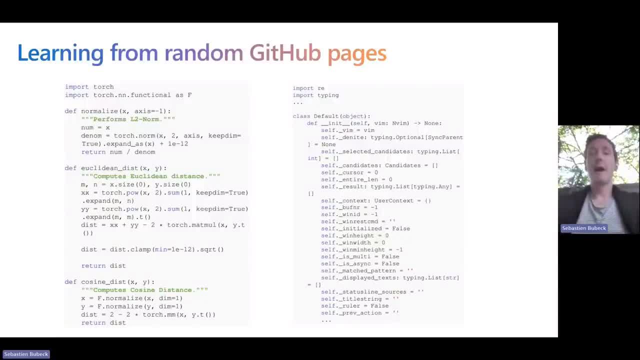 And it's hard to make sense of them in isolation. Now, you also have documents like this one on the left. 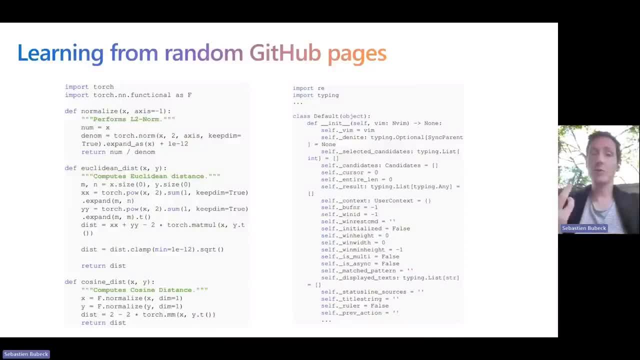 This one is much higher quality. You can learn something from it. You see that you have simple functions which are well defined. 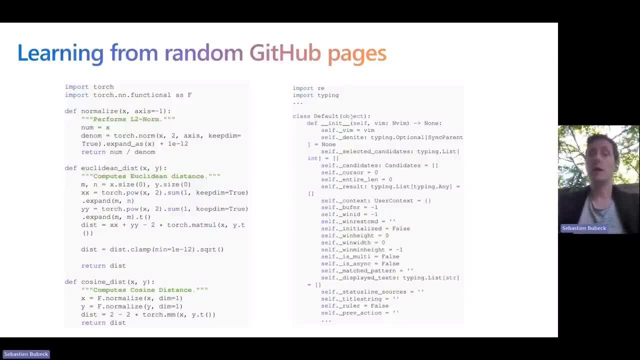 With some comments, with some doc strings that explain to you what the function is supposed to do. It stands to reason that for a large language model, it's going to be much easier to learn from documents like the left. Compared to documents on the right. Maybe with documents on the right, what you can do is merely learn some syntax. 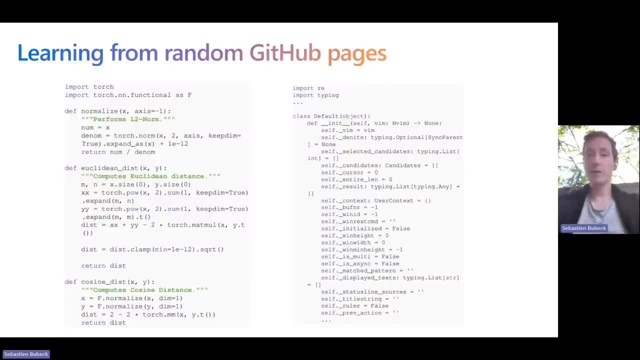 But you cannot really learn any real reason. So our idea in textbooks, all you need is why don't we focus on data set that only contains examples on the left. 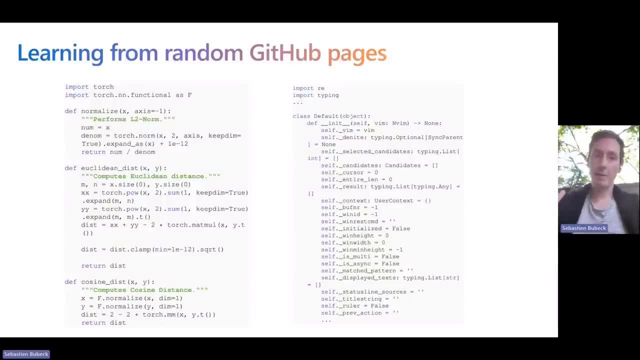 Rather than examples on the right. Why don't we focus on data that is only of textbook quality level. Okay. 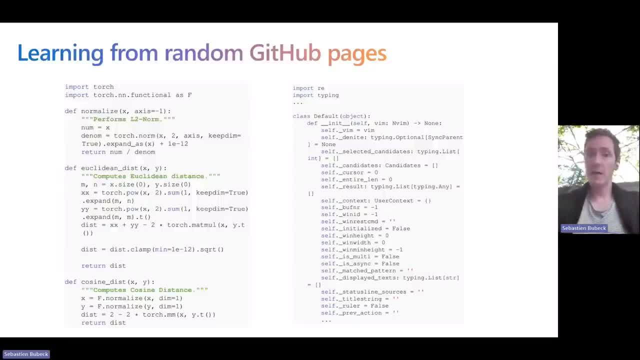 Now, how are we going to do that? How are we going to filter maybe the stack. So that it contains. So that we retain only the textbook quality. 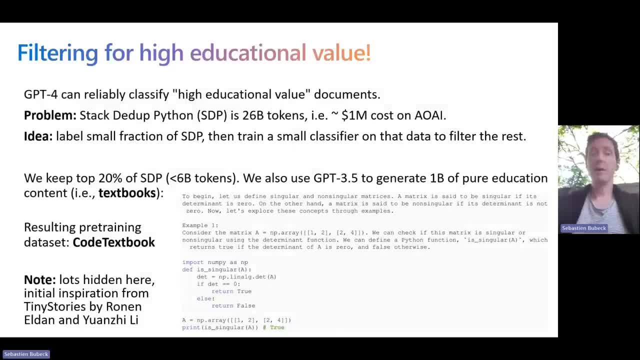 Level material. Well, we have this amazing new tool at our disposal. 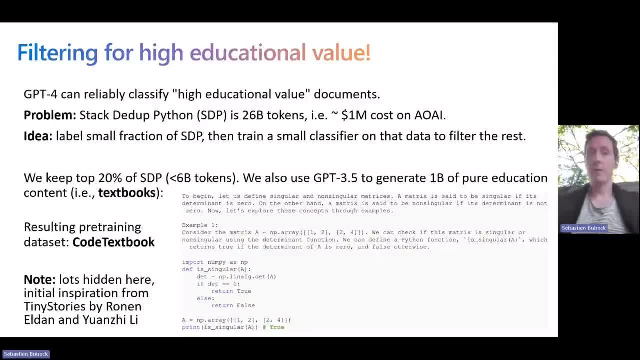 GPT-4. And GPT-4 can reliably classify high educational value. If you prompt it correctly. And you give it the two documents that I gave you on the previous slide. It will tell you that the document on the left is of higher educational value than the document on the right. Okay. 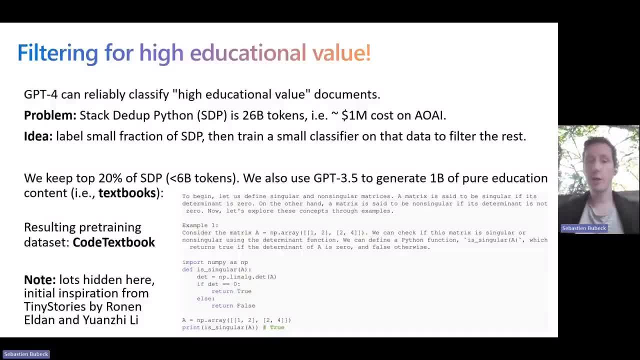 So you can use GPT-4 to get a score on how useful to teach a skill a certain document is going to be. 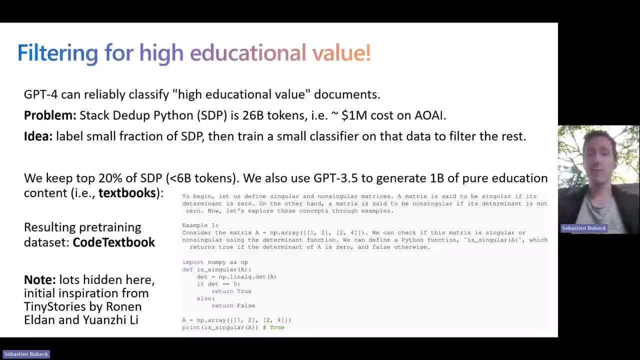 Now, here's the problem. I told you that the stack for Python is roughly 26 billion parameters. In fact, it's a stack dedupe where there is some deduplication method being applied. So let's call it SDP. So SDP is 26 billion tokens. If you were to use Azure OpenAI to label all of those documents using GPT-4, this would cost you around $1 million. Which is a lot of money. And maybe, you know, for a scientific experiment, it might be a little bit too much. But. 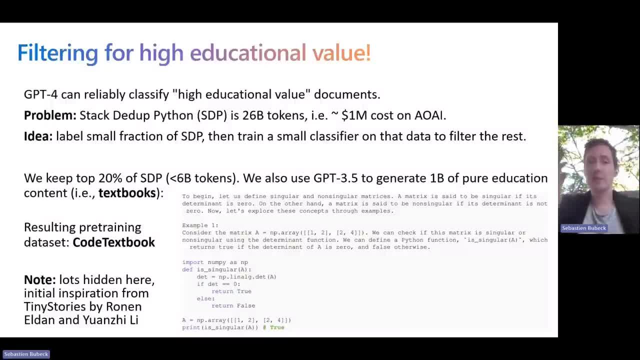 GPT-4 can do so much more than just classify high educational value document. It can do many, many things, as you all know. 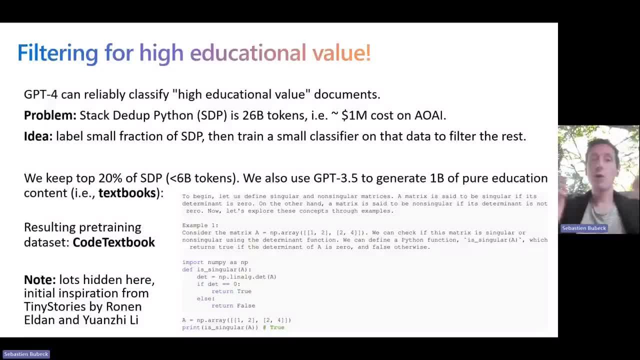 And as we discussed in the Sparx paper. So why don't we try to train a classifier that only mimics this very specific aspect of GPT-4? 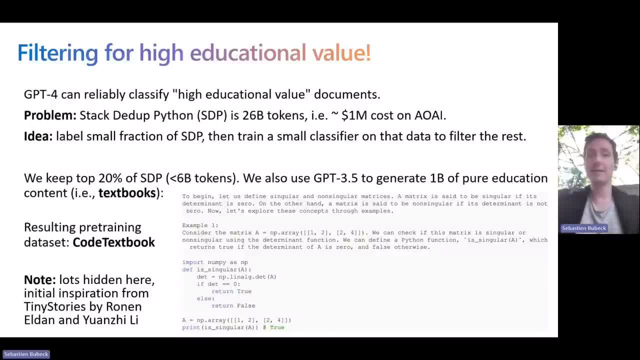 That makes sense that this could possibly work. And indeed, this is exactly what we do. We label a small fraction of SDP. And then we train another classifier. In this case, the random forest. 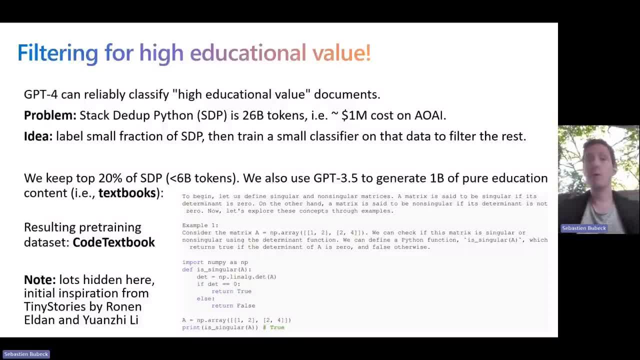 To filter the rest of the data. Where this small classifier was trained to mimic GPT-4 on the small fraction of SDP that was labeled using GPT-4. And that's basically it. 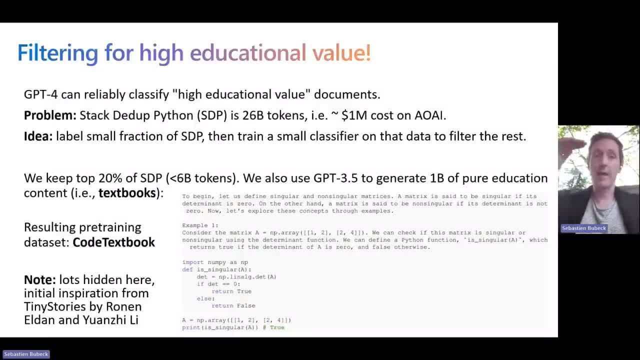 Now we have, you know, a threshold values that we can set. And we can say maybe we want to keep only the documents that have an educational value higher than 7 over 10. Or maybe only higher than 5 over 10. 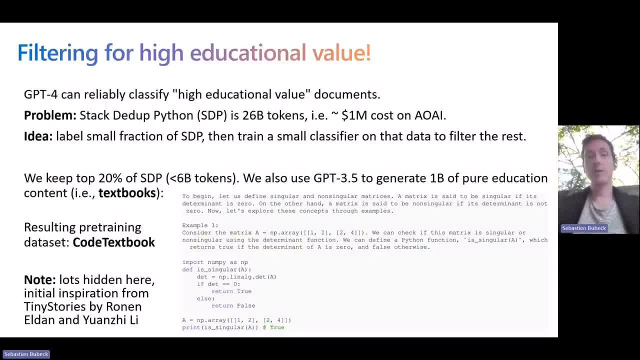 So what we decided here, you know, after lots of experimentation, is we decided to keep the top 20% of SDP. So the top 20% of SDP is only 6 billion tokens. And in addition, we also generated 1 billion tokens of just pure educational content, meaning textbooks. 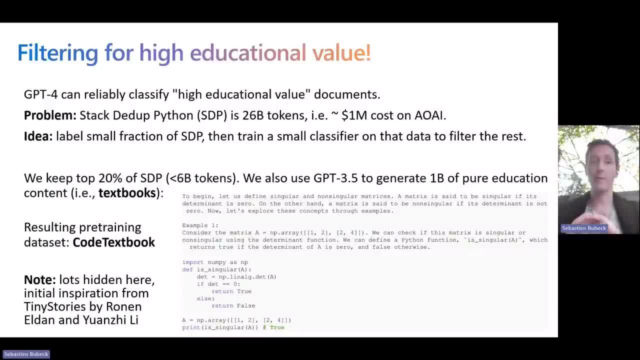 We just generated synthetically textbooks using GPT-3.5. Again, here all the magic is how do you prompt GPT-3.5 correctly to generate a lot of diversity of textbooks. 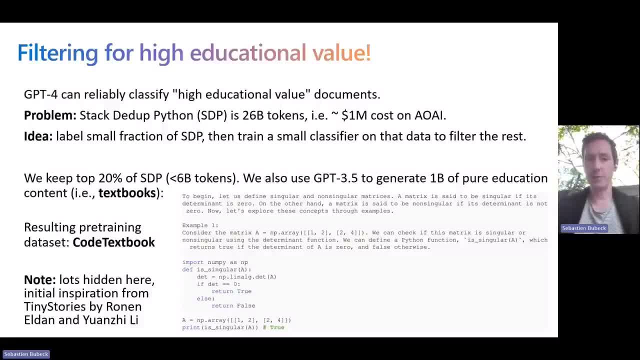 Just to give you an example, this is the type of textbooks that were generated. So you see there is a lot of natural language. Here it's talking about some matrices, defining singular values, etc. And then it's giving you an example, a snippet of code that calculates whether it's the singular values of the matrix. And then, you know, a little example. All right. I should say, so before I say that, the resulting training data set, we call it code textbooks. 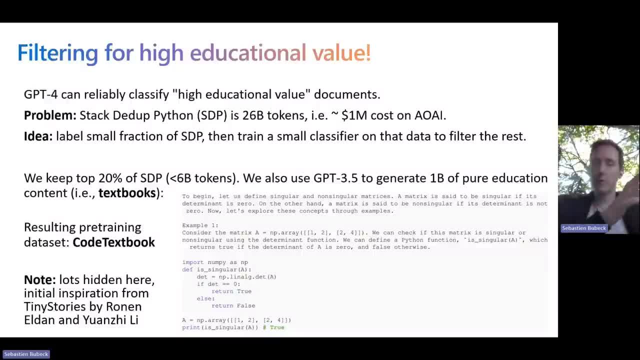 Okay, so code textbook is a combination of filtered SDP, filtered for high educational value, using a classifier that mimics GPT-3.5. 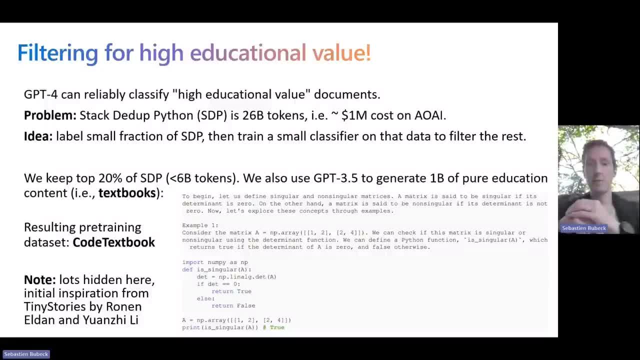 Plus textbooks that were synthetically generated from GPT-3.5. 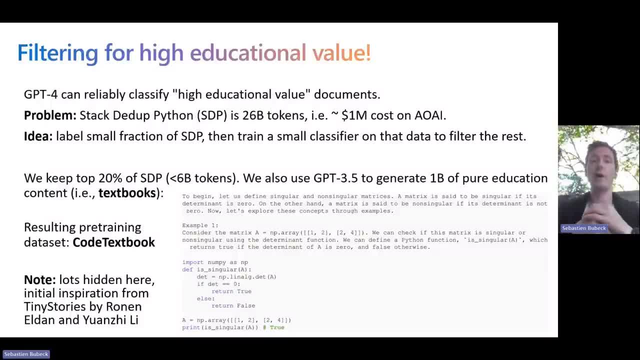 And let me say that this whole approach, this whole philosophy of creating synthetic training data, is inspired by the really pioneering work of Ronan Eldan and Yuan Zhului, 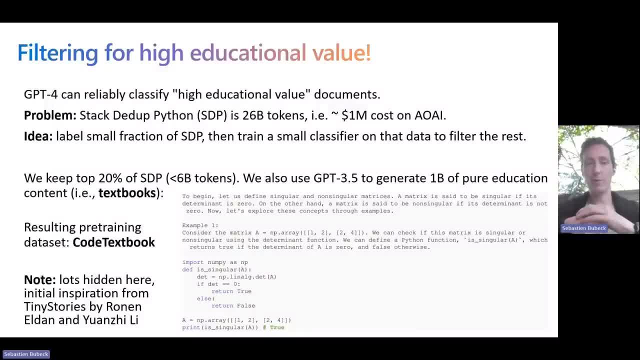 who are also part of the team for both PHY1 and PHY1.5, essential members of the team. So they created Tiny Stories. So Tiny Stories was a 10 million parameters, a model that can speak fluent English. 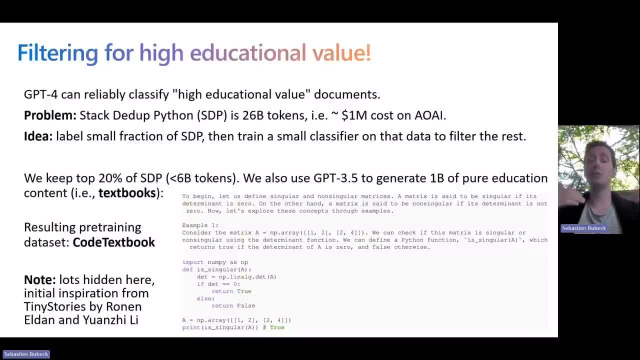 And how did they achieve that? Well, they did exactly the same thing. They used GPT-3.5 to generate a lot of stories, tiny stories, from which a small model could learn from. So what kind of stories can a small model learn from? They need to be simple enough, kind of three, four, five years old, kid type of level. So what they did is that they created a vocabulary of, you know, 2,000 words. And then they selected that random words from this vocabulary, and they asked GPT-3.5, write a story with those three words in it. And by doing that, by seeding their generation into this vocabulary, they were able to have a lot more diversity than you would get if you were just to ask GPT-3.5, hey, write me a tiny story. 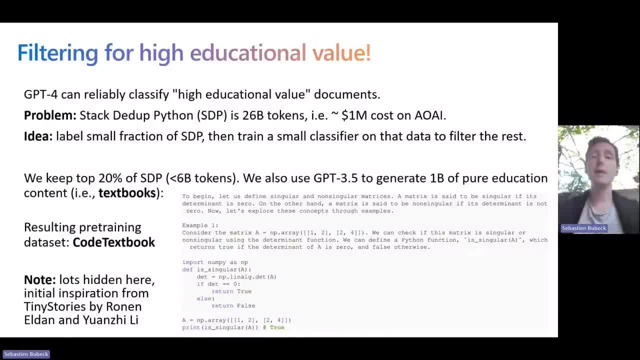 If you ask GPT-3.5 to just write a tiny story, it will over and over again write the same story about kids going to the park, you know, like their ice cream falls on the ground and they start crying or whatever, you know. 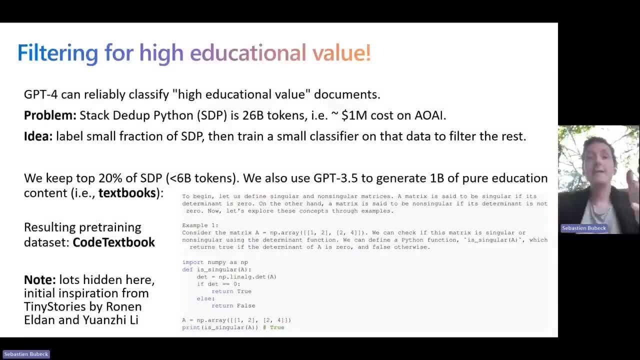 To create diversity, you need to seed the generation into some external material. What Ronen and Yuanzhu did back then was to seed it into a very simple vocabulary list. Here, for this Phi1, we have to seed it into something else. 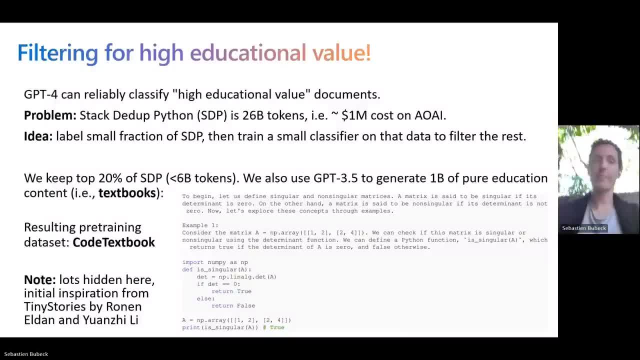 And this is where, you know, we can create a lot of diversity. 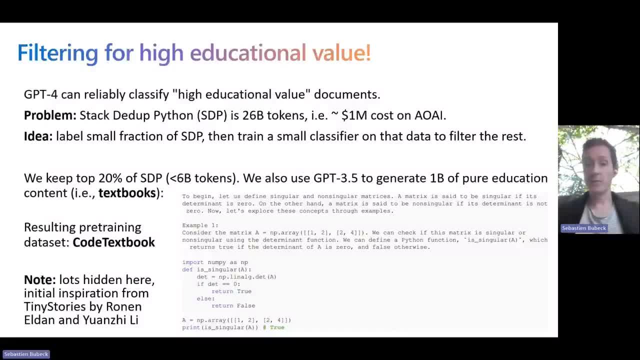 OK, so now we have this dataset code textbook. Let's see what the results are. 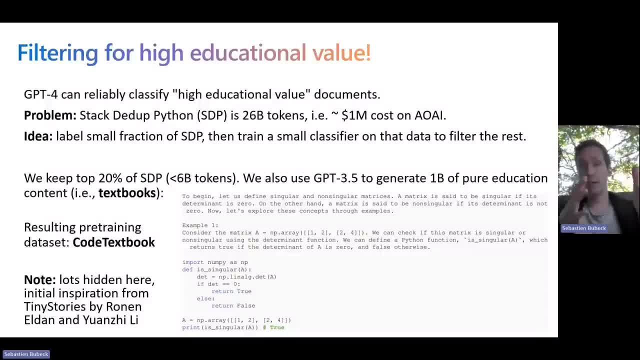 And what I'm going to do is that I'm going to compare for you what happens if you train on code textbook, which is just 7 billion tokens versus if you were to train on the stack unfiltered, the 26 billion tokens dataset. 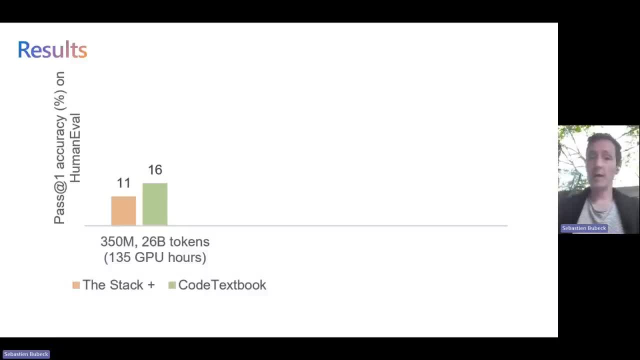 So if you do that, so you train for 26 billion tokens and let's train a small model, 350 million. You see that on the stack you get 11 percent, which is completely consistent with the tables that I showed you before. 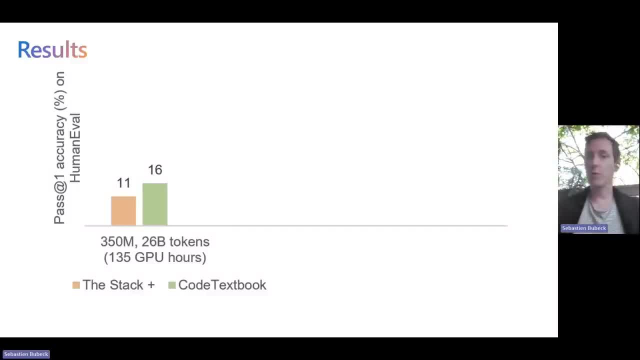 This is what CodeGen got. This is what Codex got two years ago. This makes sense, this 11 percent. You see that on code textbook, you already get 16. And note that on code textbook, we're already doing multiple passes over the data because it's only 7 billion tokens. So we're making many passes. Yet, you know, we improve. Now, as you know, there are two axes that we can scale up in deep learning. 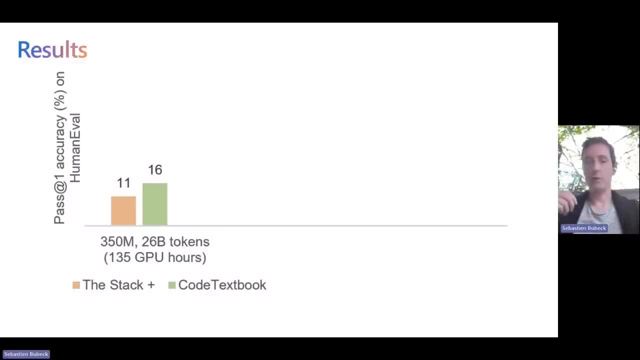 One is to make the model bigger, which, you know, we will see what happens. The other one is to spend more compute, to train for longer, to go more passes. Let's see what happens if we do that. So instead of training for 26 billion tokens, we're not going to train for 76 billion tokens. So that means that on the stack we're making four passes, whereas on code textbook we're making 10 passes over the data. And you see what's amazing is on the stack, by making more passes, you don't really improve. You go from 11 to 12. But on code textbook, because this is textbook material going over it many times, there is a lot of benefit from it. So when you go from making four passes to making 10 passes, you go at a 4% increase in human value, which is really, really significant. 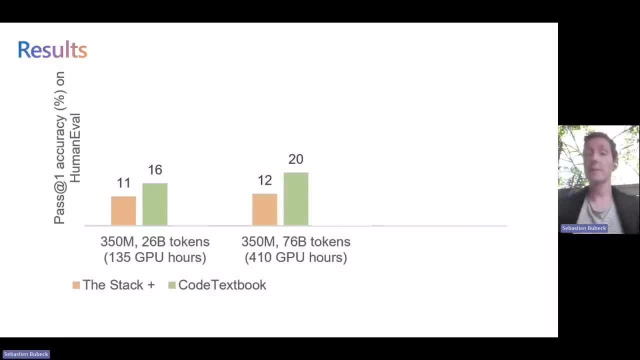 So, you know, at 20%, we're already talking about two times better than previous models at the 300 million parameters scale. OK, but what about scaling up the model? You know, maybe our data set is too small and it's not going to benefit from scaling up the size of the model. 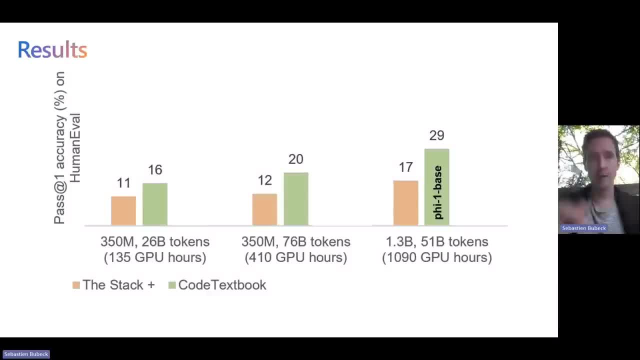 And maybe this is why those other data sets are too small. And maybe this is why those other data sets are too small. And maybe this is why those other data sets are too small. And maybe this is why those other data sets are good, because they can allow you to have a much bigger model. So let's see what happens when you train a 1.3 billion parameters model. 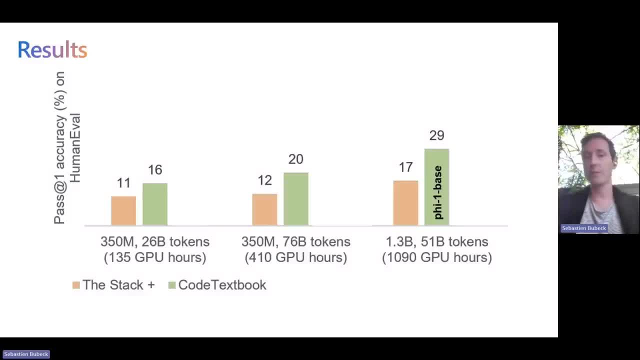 And here, of course, the magic, you go from 12% to 17% for training on the stack. 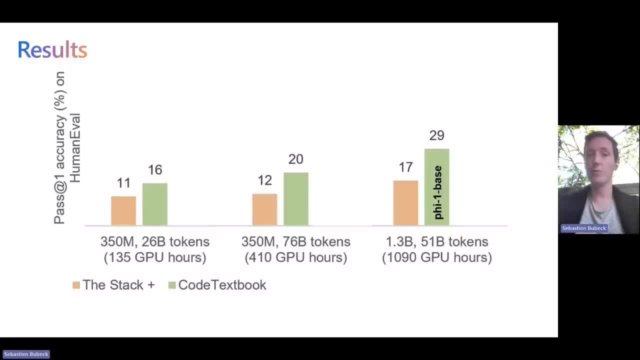 But see, you also get a huge benefit on the textbook. You go from 20% to 29%. 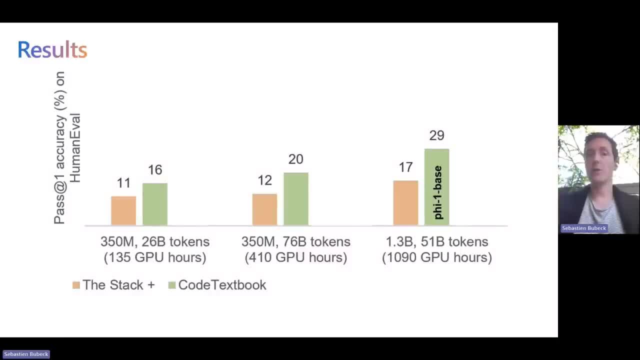 So this model, 1.3 billion parameters, trained for 50 billion tokens, we call it Phi1 base. OK, so this is our base model at 1.3 billion parameters. This is our base model at 1.3 billion parameters, 29%. 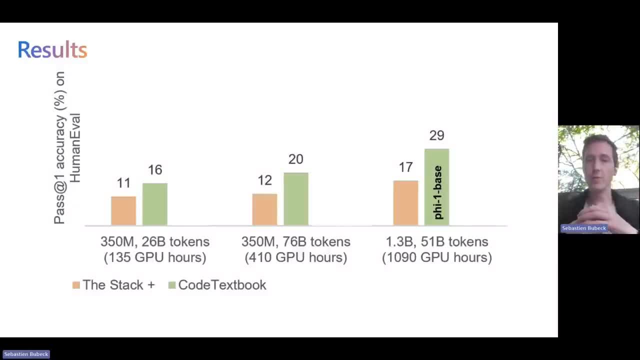 But then, as anyone who has ever tried to learn anything knows, it's not enough to just read the textbooks. But then, as anyone who has ever tried to learn anything knows, it's not enough to just read the textbooks. You actually need to exercise. You need to do some exercise. 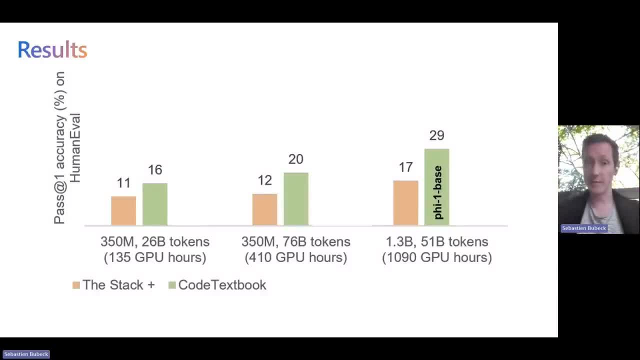 So what we're going to do is that now we're going to create an exercise data set, code exercise. And we're going to fine-tune our models on it. 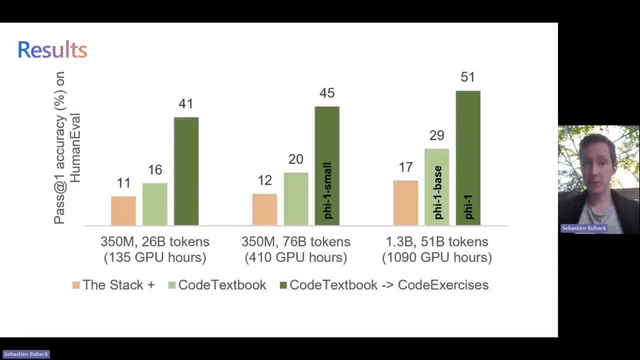 And let's see what happens. 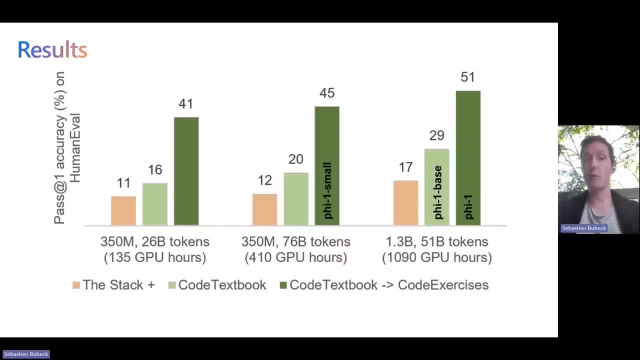 And this is where the huge jump happens. We go from... this tiny model trained for just four passes, you go from 20 to 45%. 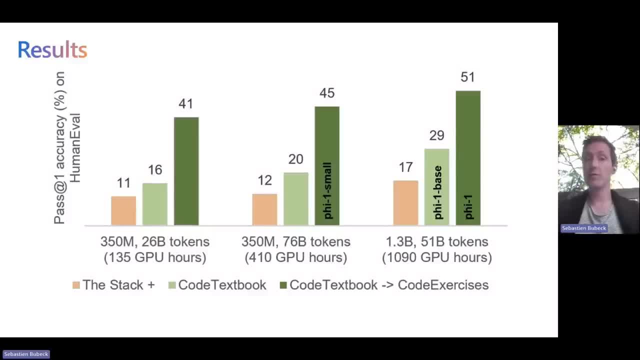 So a 45% accuracy human eval with 350 million parameters. This is close to GPT 3.5 level of accuracy on human eval with only 300 million parameters model. 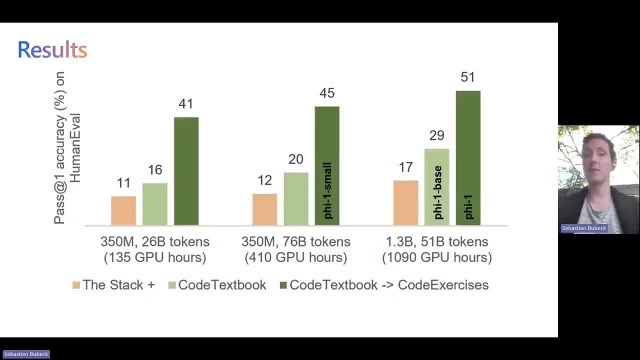 If you go to 1.3 billion, we get to 51% accuracy, and this is the model that we call PHY1. 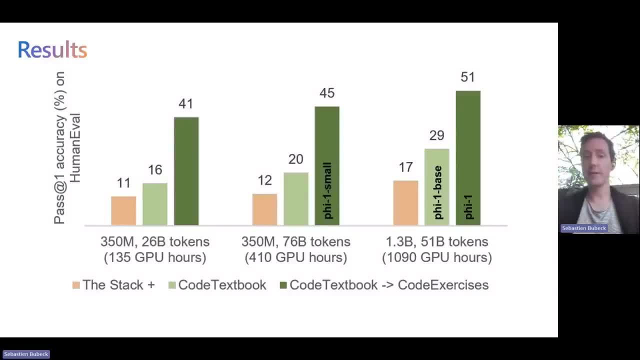 Okay, so you see some real magic happens once you fine tune on the exercises. 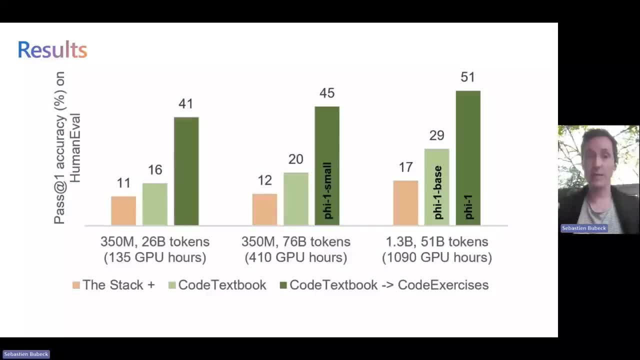 Just like for a human being, once you start to exercise and put in action your learning, 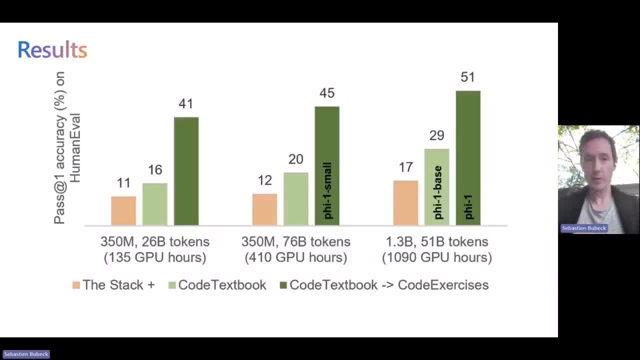 something really significant happens in your brain. So what is this code exercises, and are we cheating somehow when we train on code exercises? 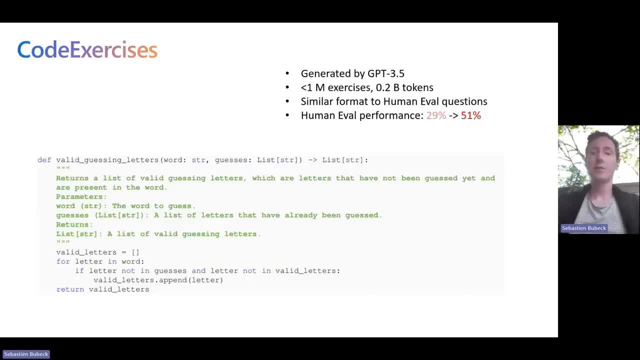 The results are so good, is something fishy going on? 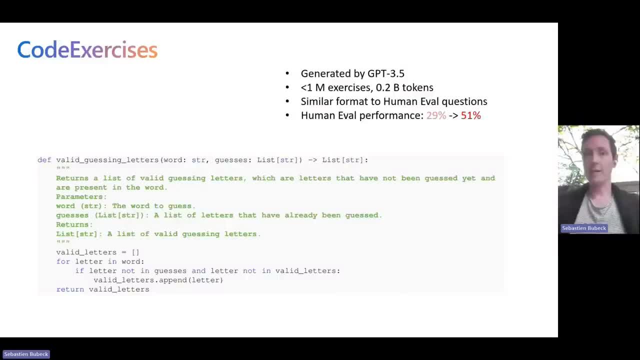 So code exercises is a dataset, a small, a tiny dataset of only 1 million exercises, which corresponds to roughly 200 million tokens. 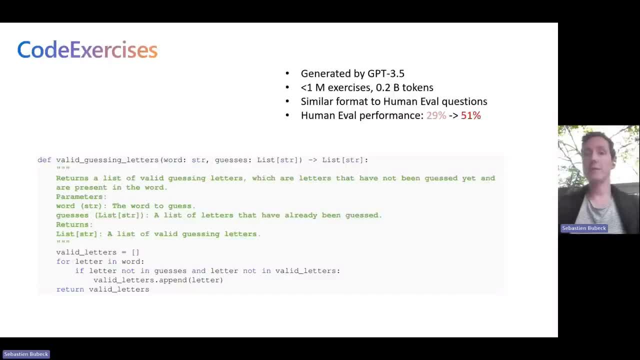 It was generated by GPT 3.5, and the format of the question is similar to human-to-human code. 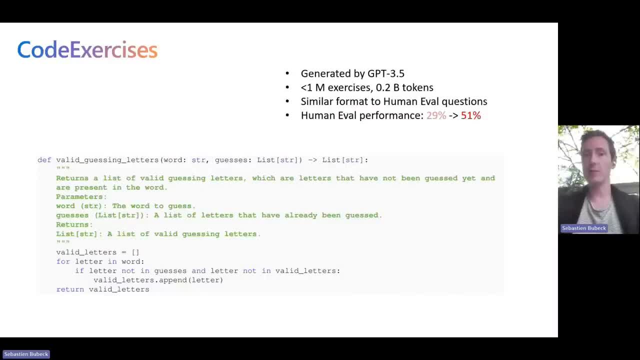 So you have a function name, you have a doc strings that tells you what to do, and then it's autocompletes, okay? 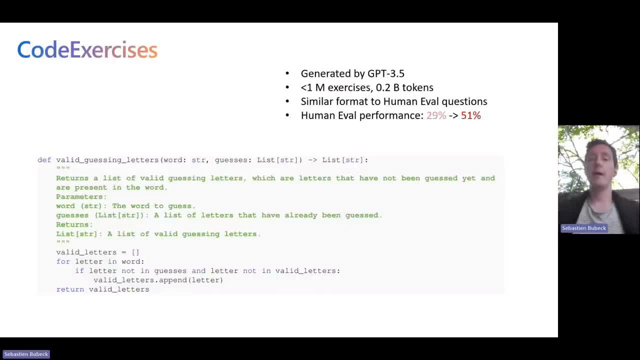 So it's very natural to ask, okay, are you cheating somehow? 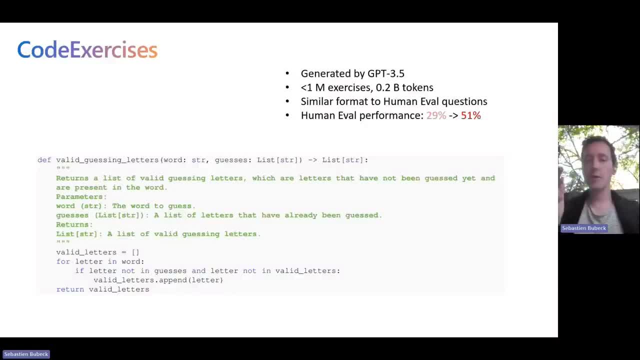 Is there contamination? Is it that maybe many of the human eval questions, 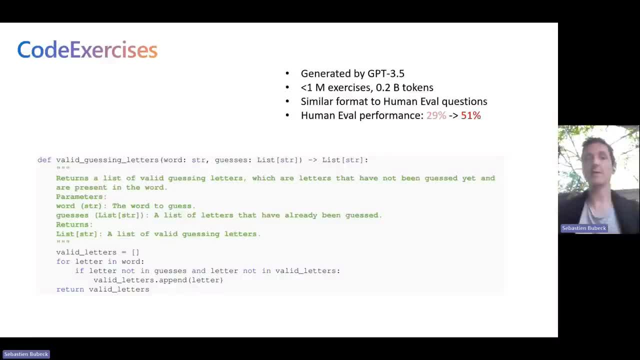 they leaked somehow and they are in your code exercises dataset? Of course, we didn't want that, but maybe it happened just because GPT 3.5 knows human eval and somehow copied those questions. 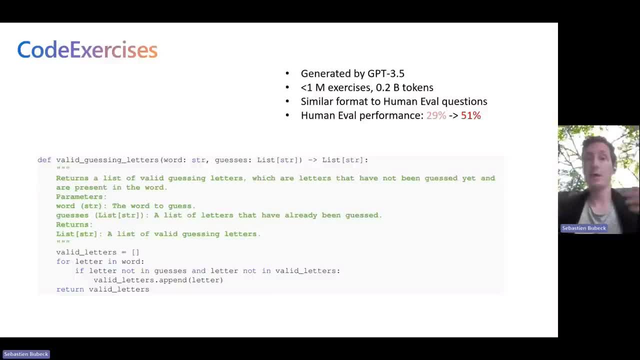 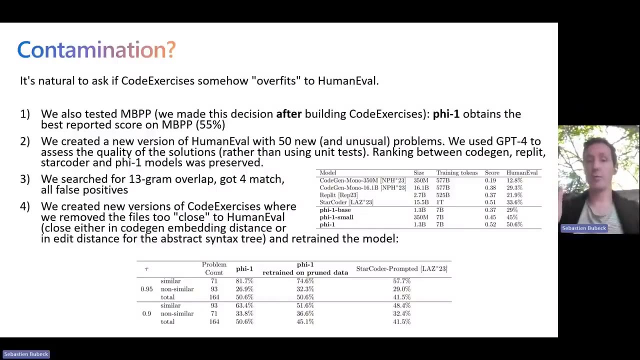 So it's very natural to ask, and it's important to ask. So let's try to answer this question. Okay, let's see if we were cheating. And it's a difficult question as many of you know. So maybe the first answer, which is a weak answer, but it's the first answer, is that we didn't just test on human eval. I just told you that we also reported score on MPPP, and there we get 55%, which is even higher than other models. 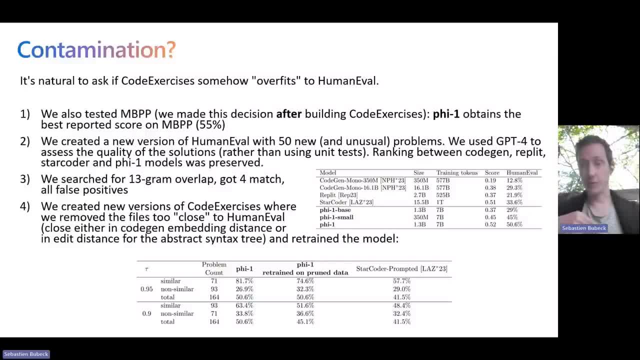 So if anything, maybe we're not overfitting to human eval, because on this test, we're just testing the human eval. So we're just testing the human eval, and we're just testing the human eval. 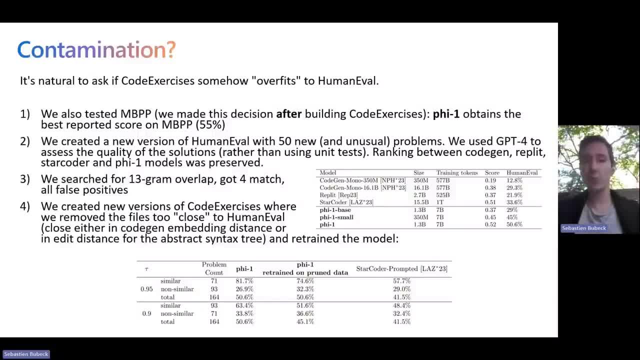 And these other benchmarks were doing great. Now, of course, you know, maybe we're overfitting to both human eval and MPPP. I mean, who knows? Okay, so this is not enough of an answer. 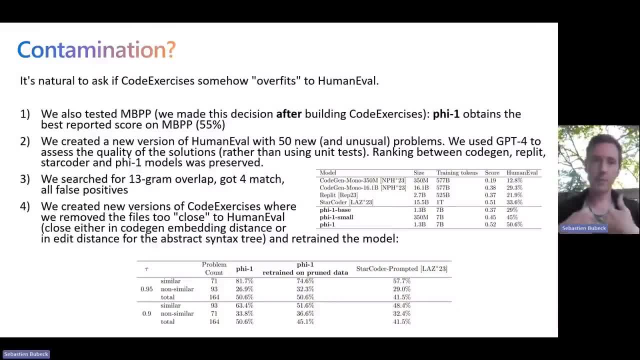 A second answer, which I find very convincing, but for this answer, you need to kind of trust us, because we didn't fully release all the details. But we had in our team a sub-team, which was separated from the team creating the training data. And this separate team created 50 new problems, 50 new human eval-style problems, but highly unusual, really of a different style, okay? And we tested our models and all the other models on these 50 new questions as kind of an independent test of understanding. 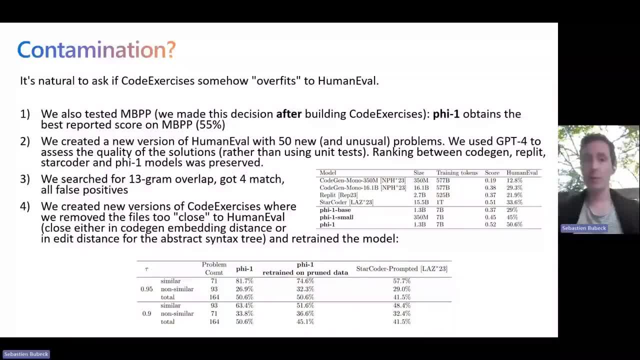 And instead of using unit tests, we used GPT-4 to assess the quality of the solution. 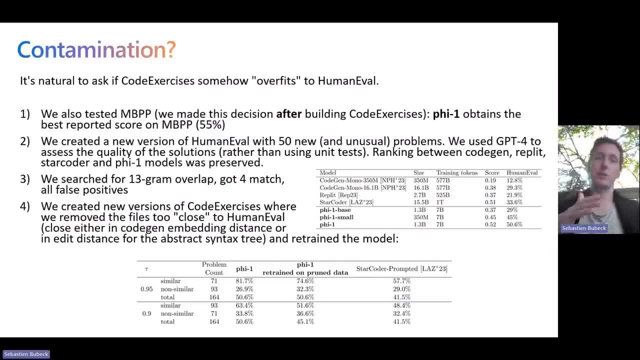 Why did we do that? Well, there is a cheap answer, which is just so that we don't have to write unit tests. But also, GPT-4's evaluation is very interesting, because it's able to create, it's able to grade a solution, even if the solution does not really work. 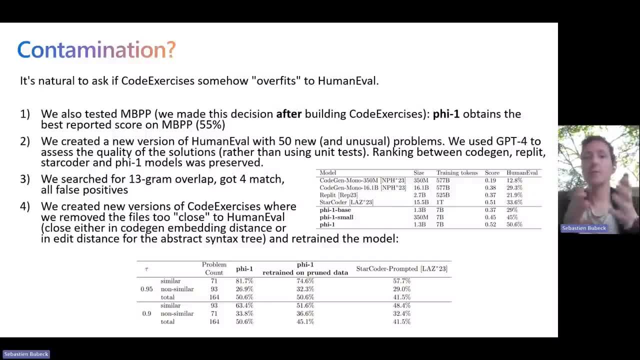 You know, just like a student can come to you and their code is not working, but they are going in the right direction, 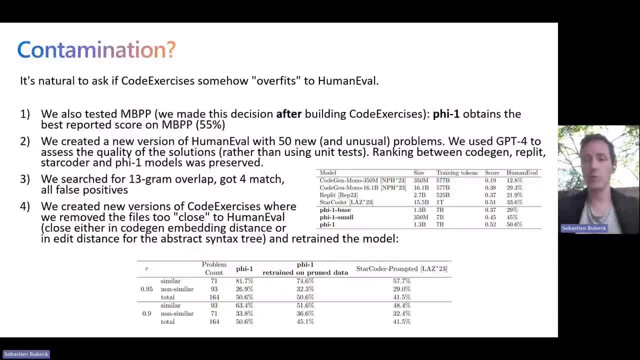 and you can still grade them and give them some points, even though, you know, the thing is not running exactly like you wanted, 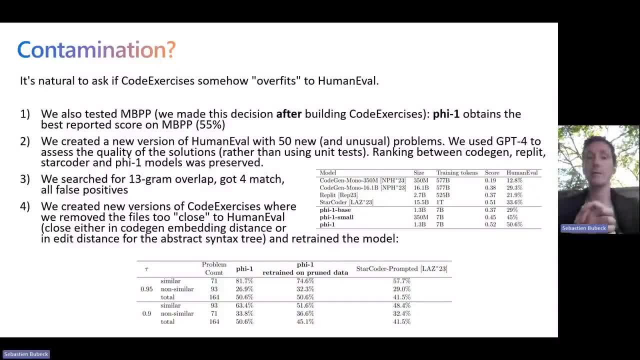 it's the same thing. GPT-4 can grade whether the models are going in the right direction. 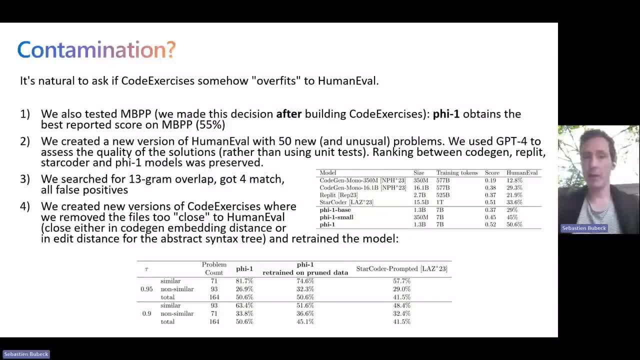 So we tested CodeGen, Replit, StarCoder, and our PHY1 model, 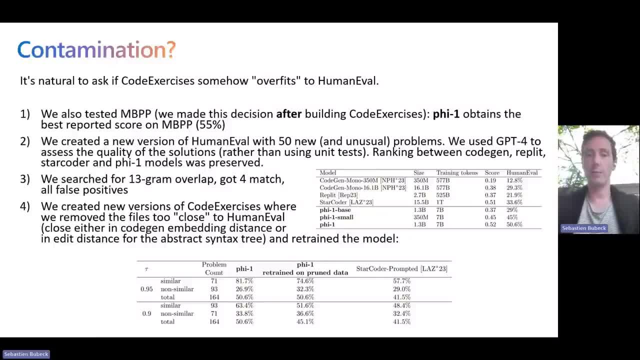 and these are the scores on this new 50 new problems. So this is a very interesting exercise. And you see that the ordering is exactly the same. So you see PHY1 base gets 37%, PHY1 small 45, and PHY2 52%. So the ranking is exactly the same as the human eval ranking. 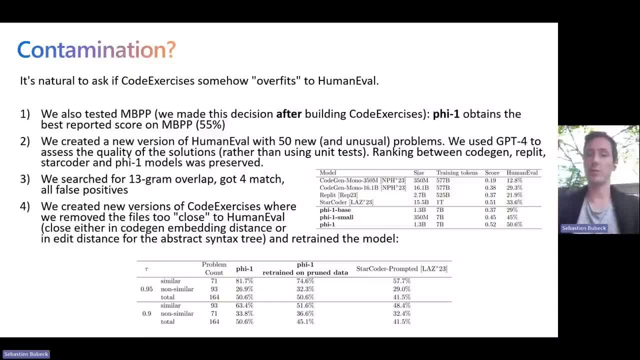 We see that PHY1 is roughly of the level of StarCoder, which is what we expected, and it's much better than to CodeGen. 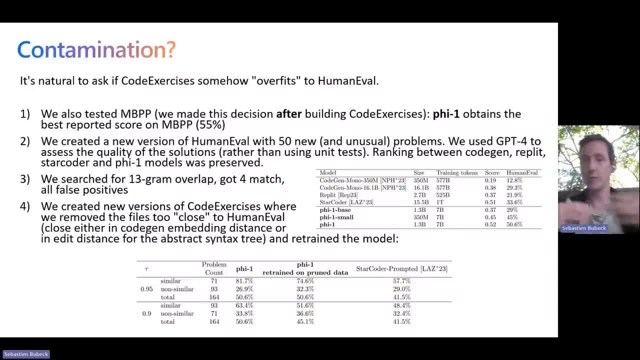 Okay, so I find this personally very, very convincing. Of course, you have to kind of trust us for this. 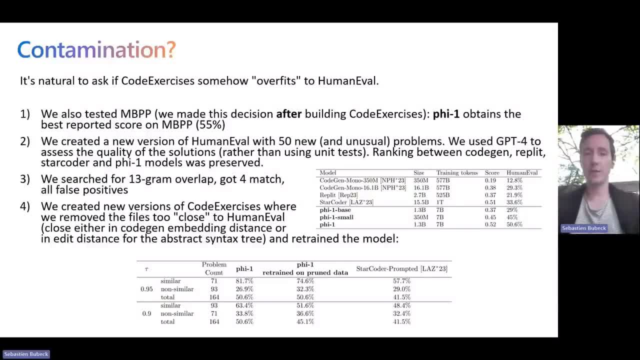 So let's go, let's go over some other contamination tests where maybe you have to trust us less. 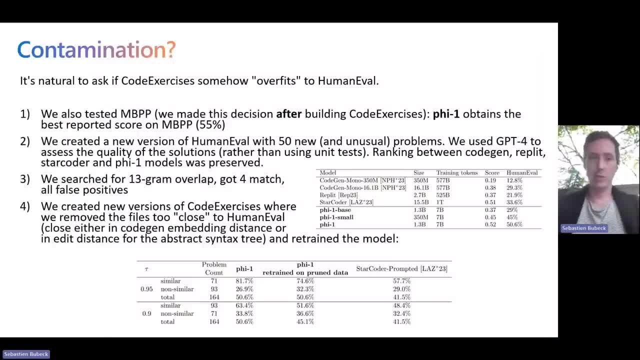 So one standard thing that people do in the community, which I don't think is enough by any means, but this is just to show you that, at least on the standard way to test for contamination, we're doing great. We searched for, you know, little n-gram overlap, and we searched for 13-gram overlap and got four matches between human eval and the code exercises dataset. Turns out that those four matches were actually false positive. 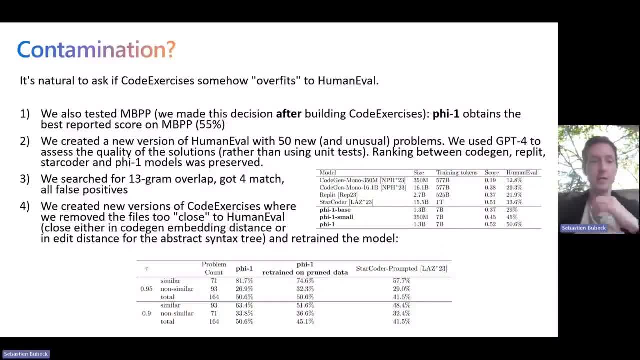 It was just some random substring that was matching. It was not at all the same exercises. 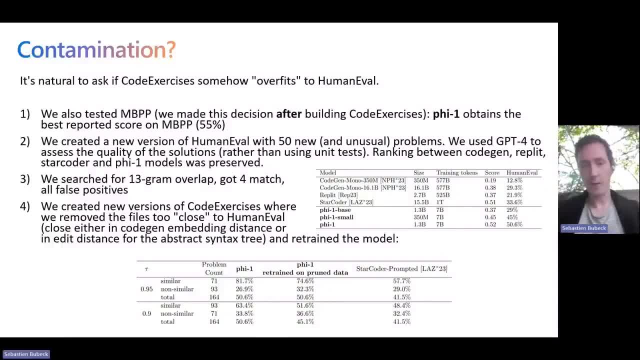 So at least there is no exact copy. Okay, but of course that's not, that's not enough. 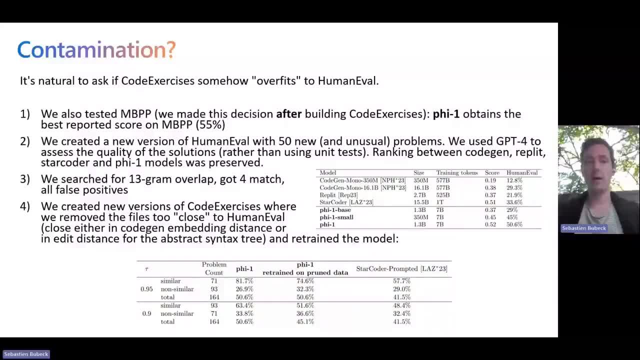 So let me go over the last contamination test that we did, which I think is a really good one. 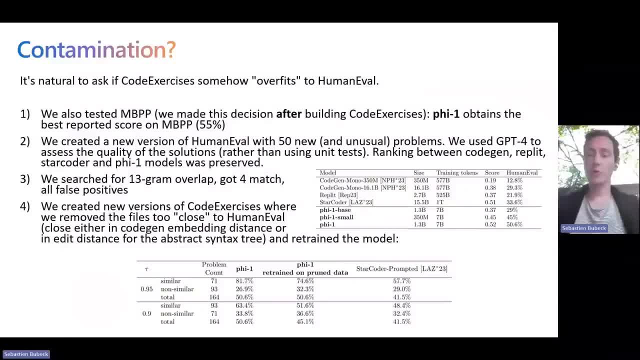 So what we did is we looked for all the files in code exercises that were close to anything in human eval. And here's the notion of closeness that we used is close in either the CodeGen embedding, so you can use CodeGen to embed, you know, a human eval code, and then you can test the difference between the human eval code embedding and an embedding of a document in code exercises. 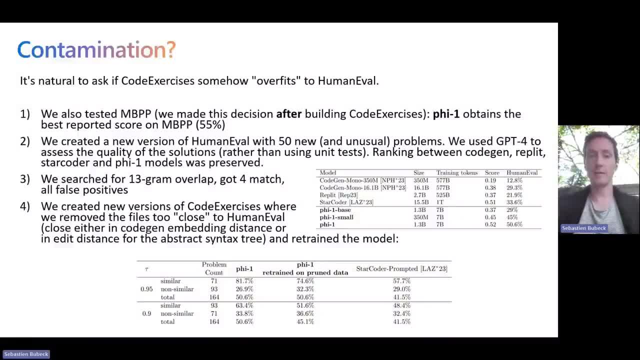 And we also use the edit distance in the abstract syntax tree. And for the edit distance in the abstract syntax tree, we varied various thresholds. You know, you can look at, are you 95% close? Are you 90% close? And even, you know, 95% close is already not very close. Just, just to, to, to be able to understand it more publicly. 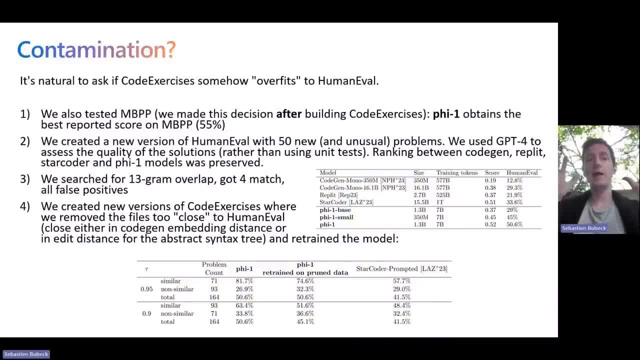 And now what we did, it will take just a few minutes to understand exactly what we did. 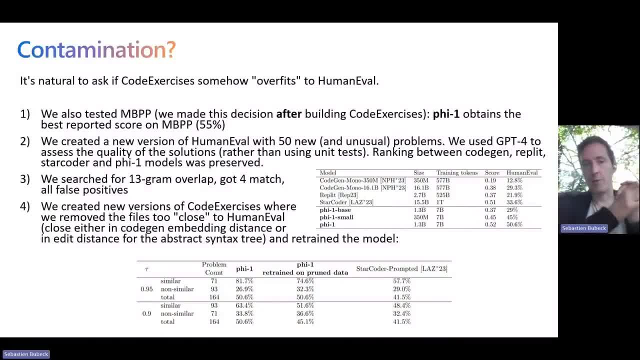 What we did is we looked at all the similar document encode exercises, similar to anything in human eval. And then we removed all of those similar document encode exercises and retrained the model and tested the performance. 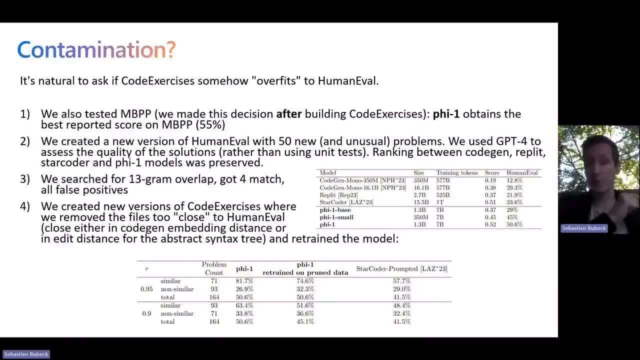 And not only that, but we also tested the performance on the subset of human eval that was deemed similar and the subset that was deemed dissimilar. 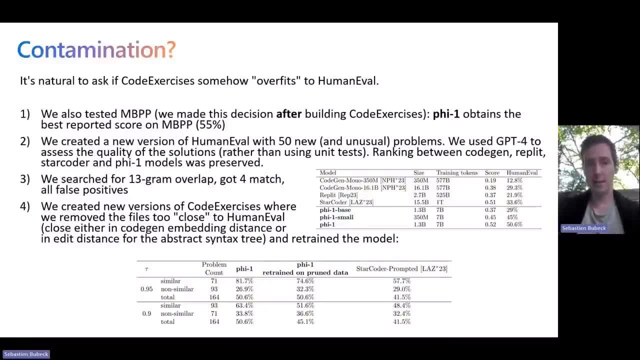 let me give you the rundown. Tau is the threshold for the abstract syntax tree edit distance, so either 95 percent or 90 percent. Again, we're dividing the human-eval problem into those that were deemed similar to some document in code exercises, and those that were deemed non-similar. 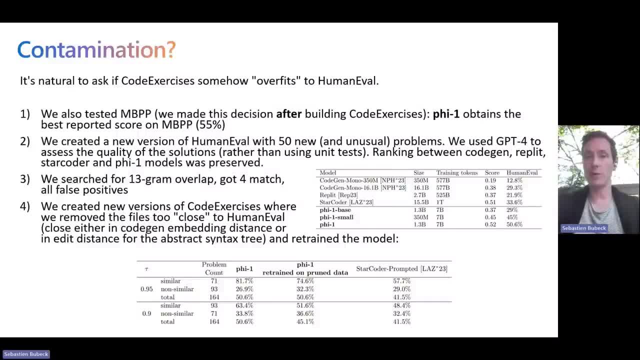 You see at 95 percent, 71 problems out of the 164 problems were deemed similar. 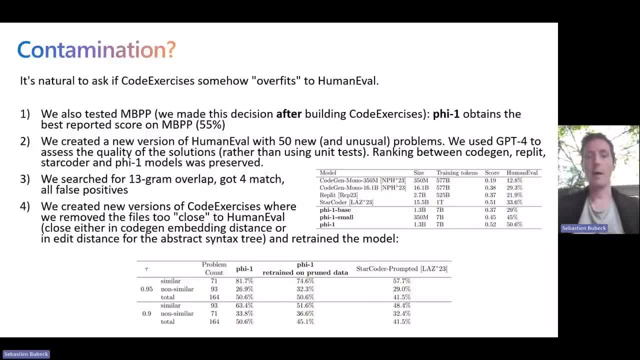 At 90 percent, of course, there were more. It's a more lenient threshold. 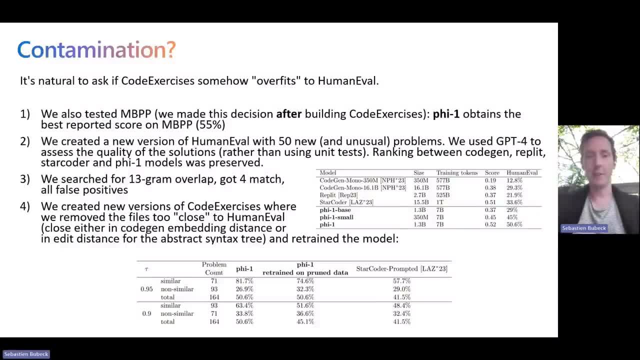 We got 93 problems that were deemed similar. Now, let's look at Phi1 accuracy on those subsets. 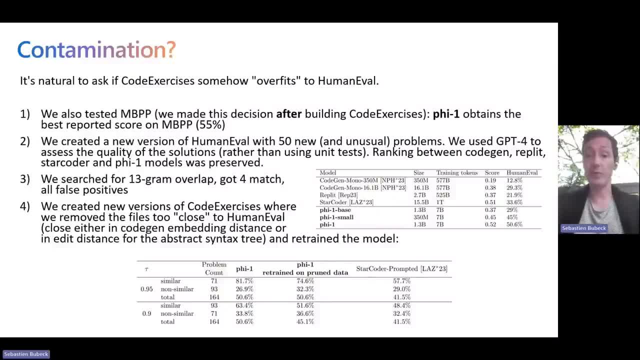 You see that Phi1 accuracy on the problems that were deemed similar is 81 percent. So very, very good, which makes sense. There are similar problems in code exercises, so it's doing very well. 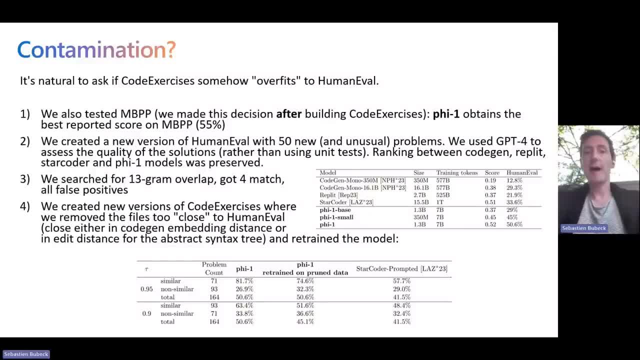 On the non-similar, it's doing much worse, 27 percent. Here is the key point. 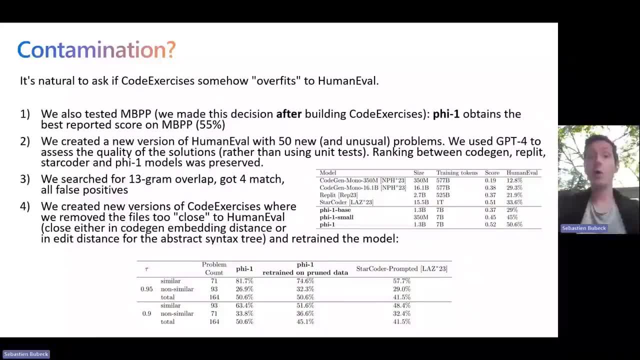 What happens when you retrain Phi1, but you prune all of the documents in code exercises that are deemed similar to anything in human-eval? 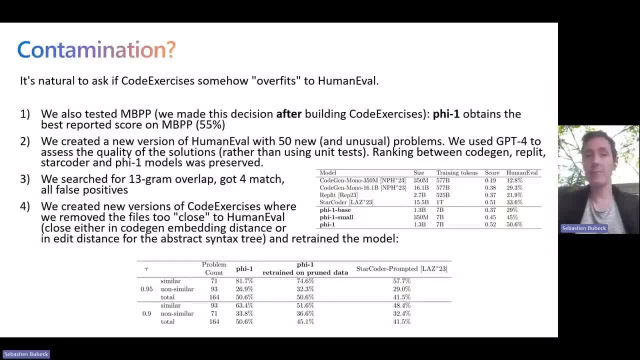 Of course, the accuracy on the similar problem goes down, but not by much. This is the key point. 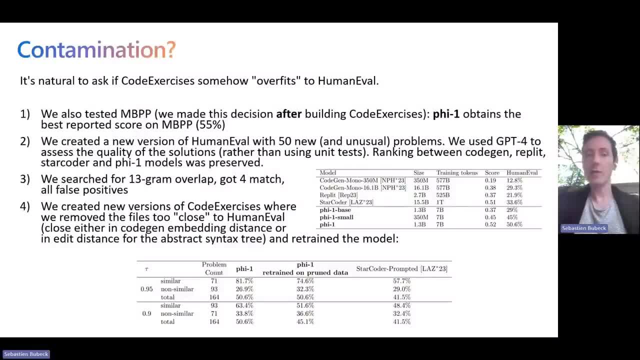 It goes down from 81 percent to 74 percent. What about the dissimilar? The dissimilar, it even goes up. 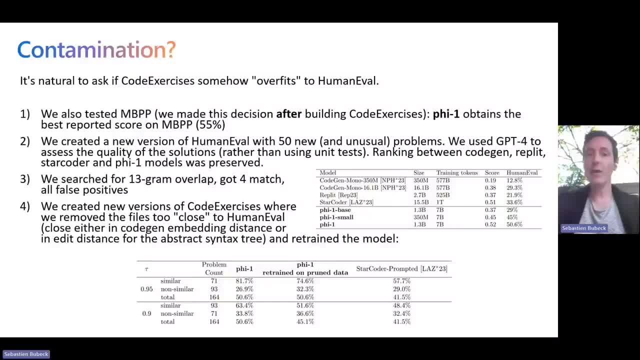 You go up from 27 to 32 percent. So in fact, the overall accuracy stays the same, even though you have pruned a lot of data. 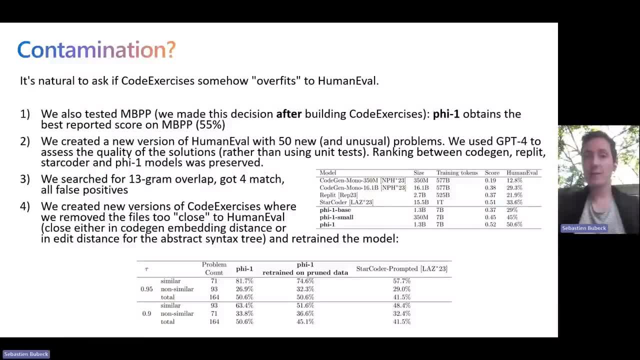 What's more is that you still are better than StarCoder on all the subsets. StarCoder is 57 percent on the similar and 29 percent on the non-similar. Why is, by the way, StarCoder also better on the non-similar, even though a priori has nothing to do? Well, it's probably because those similar problems, those problems in human-eval that are similar to some problem in code exercises, these are probably the frequent type of question, the frequent and easy type of question. 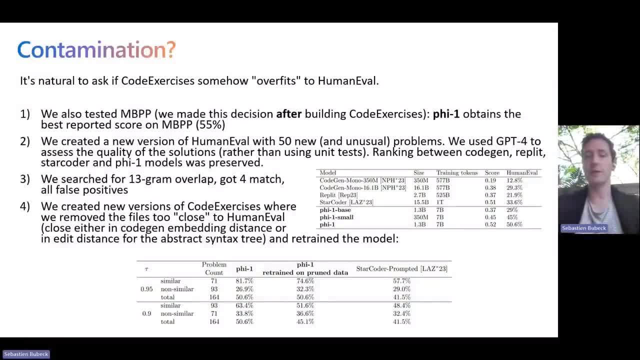 Those questions, basically every model is going to get correct, and it's more on the non-similar that it's harder. 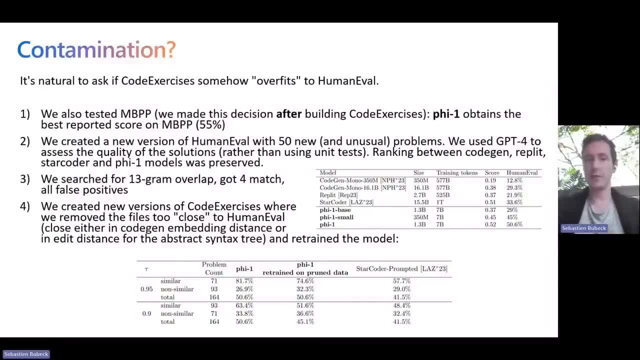 Okay. So I think this is very convincing evidence that there is no contamination at all by human-eval in code exercises. But at the end of the day, this really doesn't tell you the full picture. 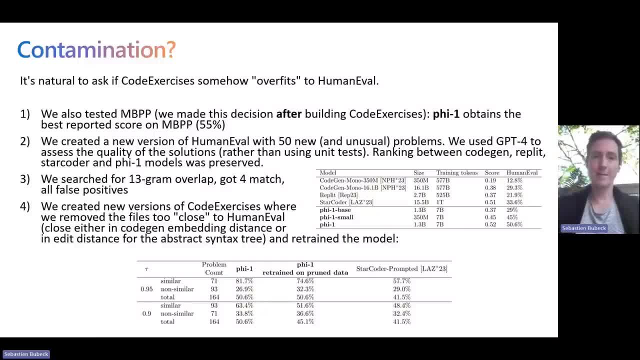 These benchmark numbers, as you all know, we are past these benchmark numbers. 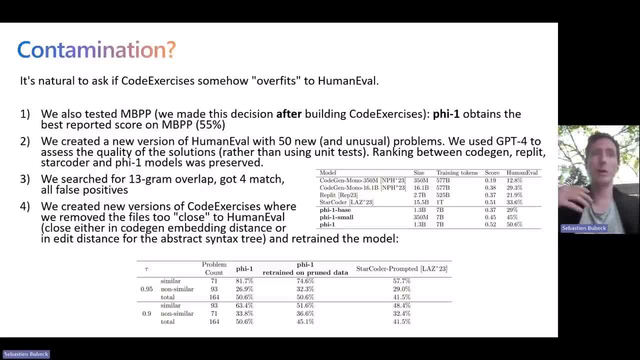 Really, what matters is when you play with the model, when you experiment with the model, what is the field that you get? This ties into this concept of emergence. 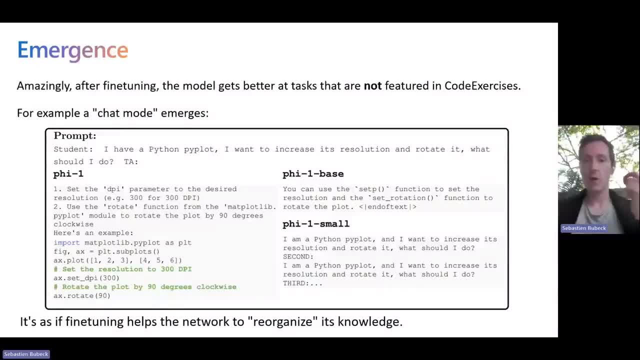 Here, the amazing thing is that after fine-tuning on code exercises, we see incredible emergence. 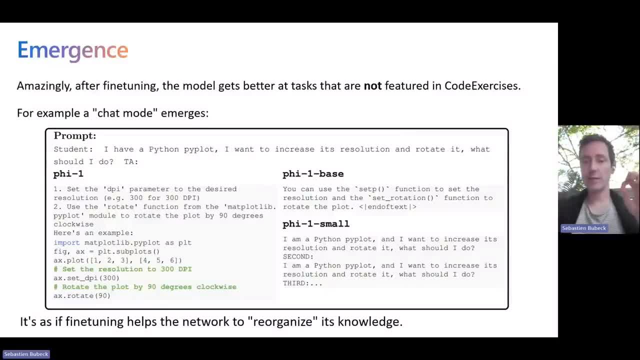 What do I mean by that? I mean that after fine-tuning on code exercises, suddenly the model is able to do things that it wasn't able to do before, even though those things have nothing to do with the fine-tuning dataset. 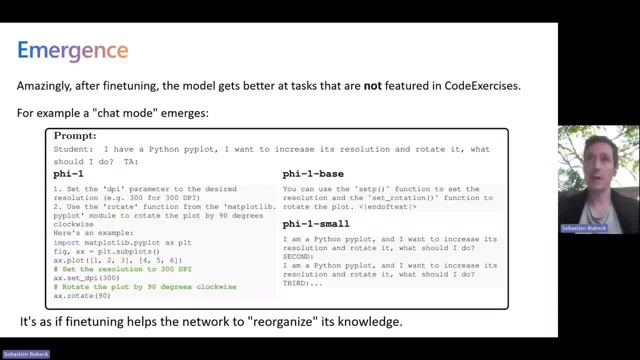 For example, there is a chat mode that emerge, which is kind of crazy. So let me give you the example. 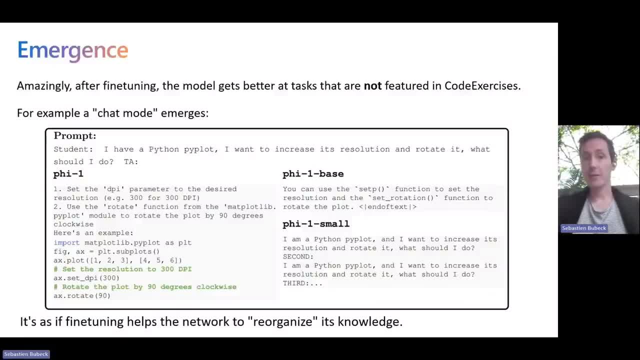 Let's say, here's my prompt. There is a student saying, I have a Python and PyPlot. 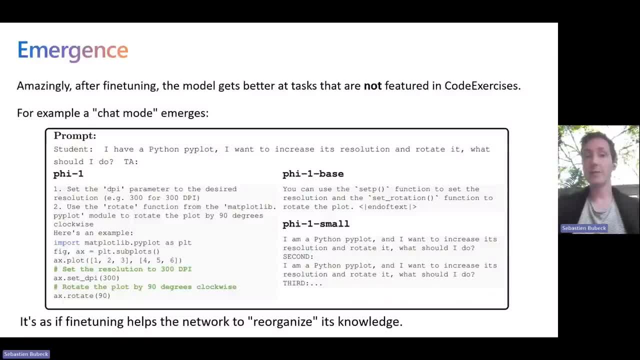 I want to increase its resolution and rotate it. What should I do? Then the TA replies, with Phi1, which has been fine-tuned on code exercise, set the DPI parameter to be the desired resolution. Use the rotate function, blah, blah, blah. 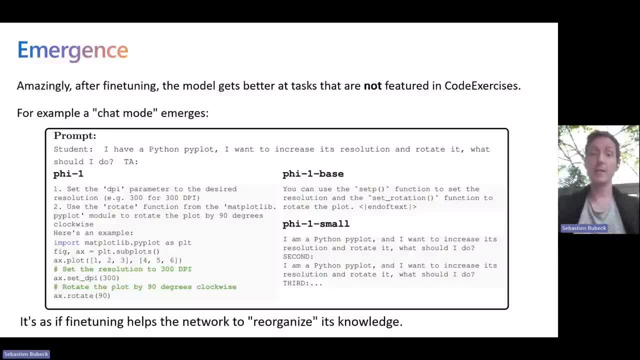 Here's an example. The TA is explaining to you what to do. 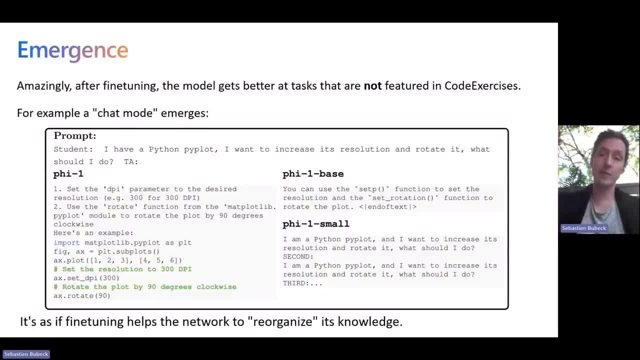 This has nothing to do with code exercises, where code exercises is just definition of a function, doc string, and the function. What does Phi1 base? Do on this question, Phi1 base does much worse. So Phi1 base is not able to basically summon the right knowledge inside the network to answer this question. Because where is this knowledge coming from? Of course, this knowledge is coming from the textbooks, the synthetic textbooks that we trained on. So Phi1 base has been trained on the textbook knowledge that is needed to answer this question. 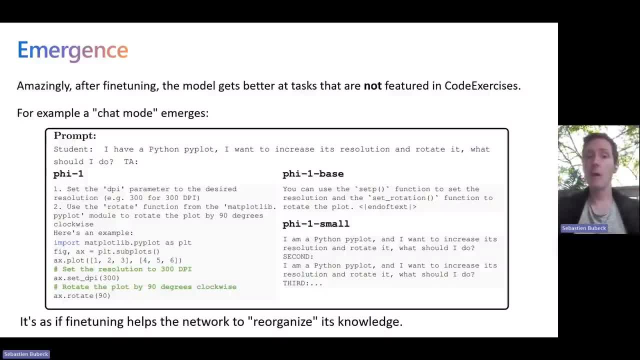 But it's not able to do it, but Phi1 is able to do it. Why is that? 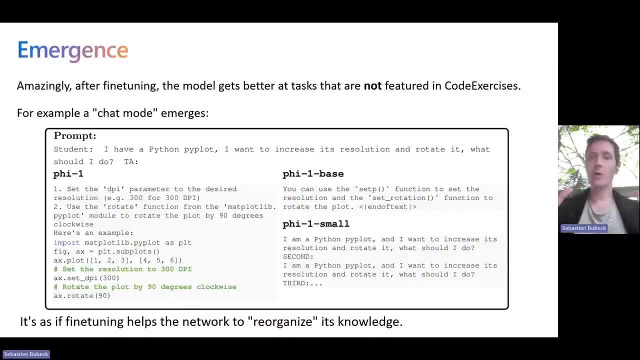 It's as if the fine-tuning, it helps the network to reorganize this knowledge. It's able to, by fine-tuning on the exercises, the model cleans up itself. 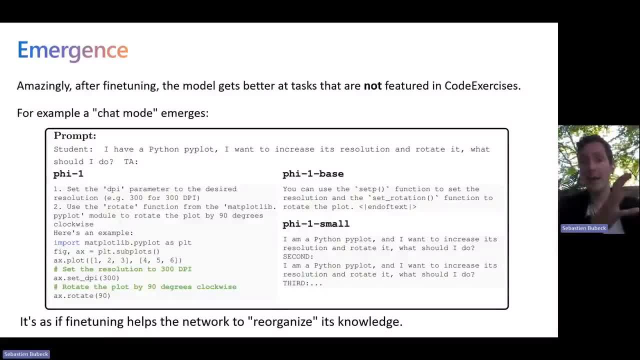 It removes all kinds of junk, so as to focus on the things that really matter. 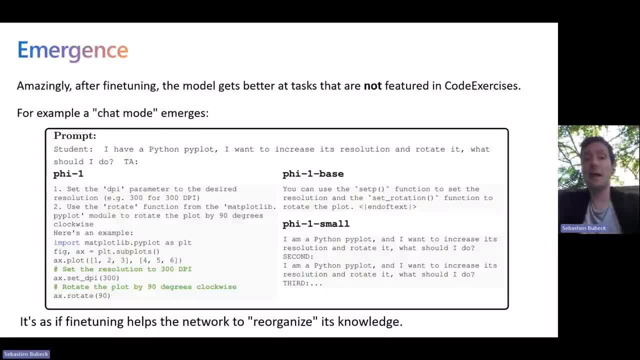 By doing so, it also makes all interesting elements from the pre-training data surface back. 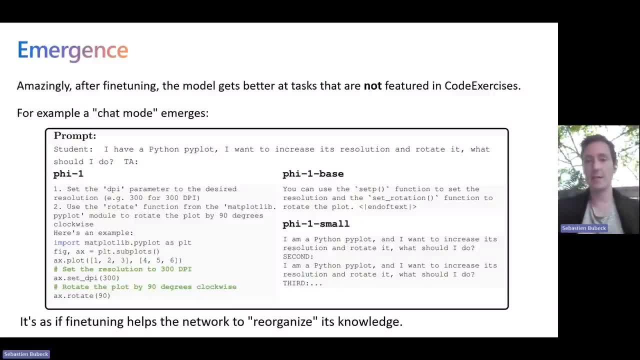 So this is really, I think, much more convincing than any type of benchmark numbers. 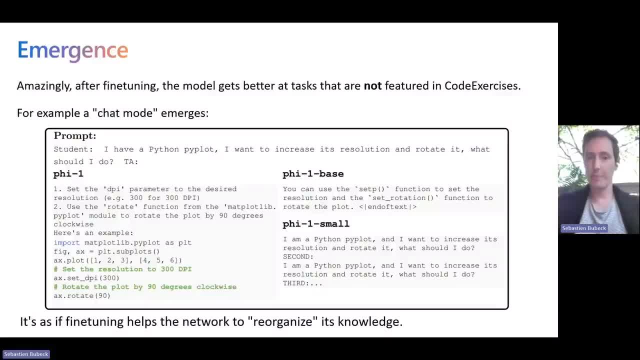 So in the last, 10 minutes or so, what I want to do now is to tell you about our next step that we took, which is creating Phi1.5. 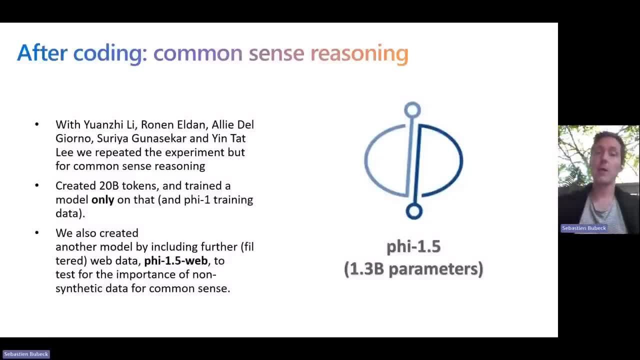 So Phi1.5 is, we try to apply the same recipe, but instead of going after coding, we went after common sense reason. 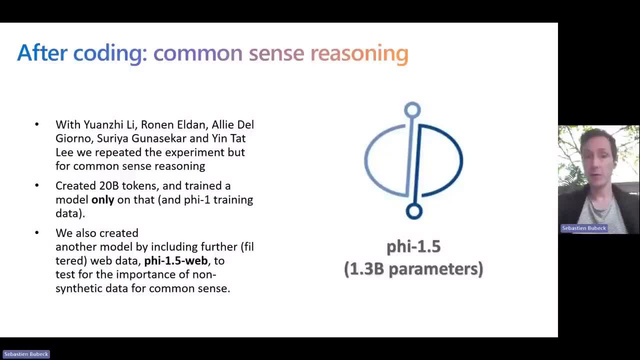 This was done with a smaller subset of the team, Yuanzhu Li, Uledi Effort, Rondan Eldan, Ali Delgiorno, Surya Gunasekar, and Yintat Li. 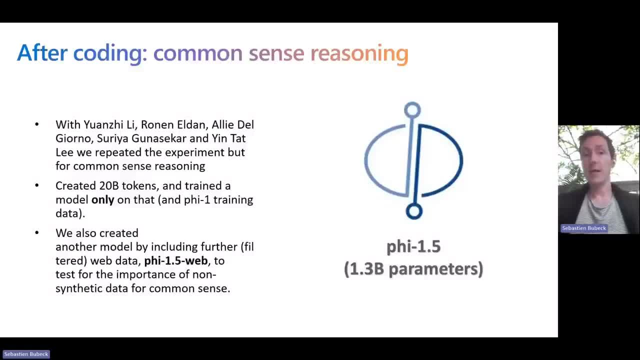 Now, what we did is that we created 20, a billion tokens, so much more than before, and we trained the model only on that. 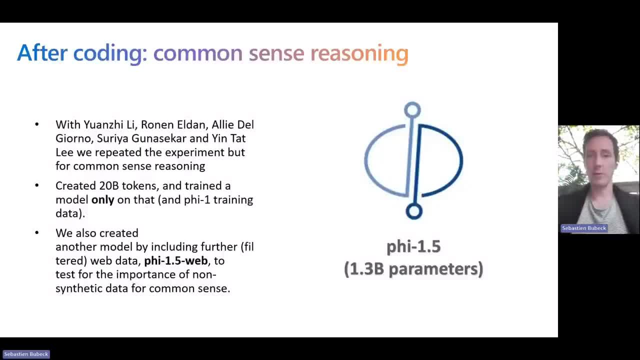 Only on that plus the Phi1 training data that we had already created. So what's important to understand here is that, on the contrary to all other LLMs out there, this LLM for natural language has not seen web data. 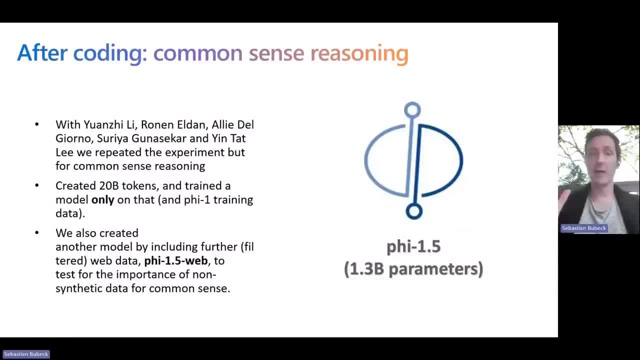 It has not been trained on web data. It's trained on completely different style of data, which is our synthetically generated textbook to teach common sense reasoning, 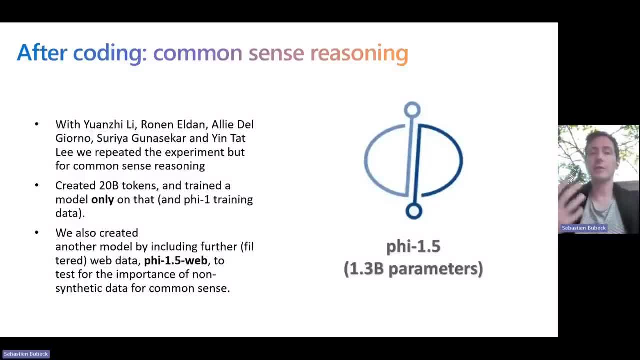 and world knowledge. So you can already imagine that it's going to be a quite different field. 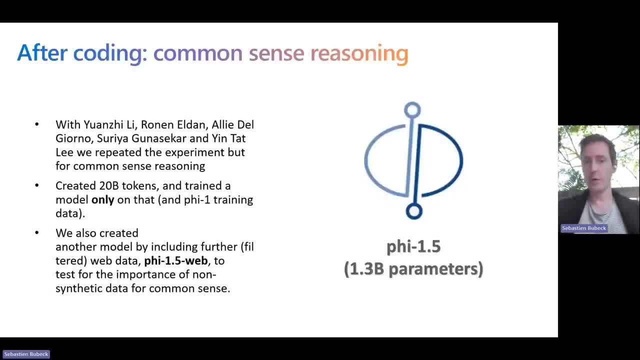 Now, to test for the importance of web data, we also trained another model, which was enhanced further with more web data, filtered web data. 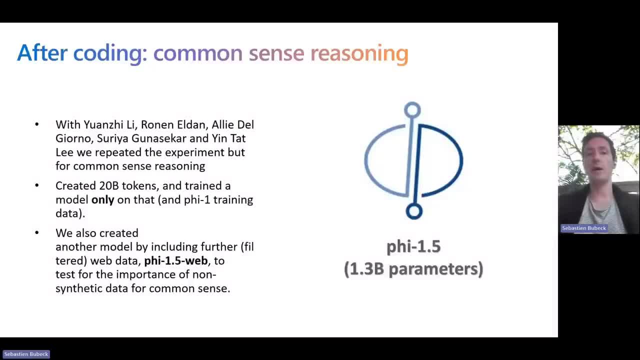 So we applied the filtering techniques that I told you about before to the Falcon dataset, and doing this, we created Phi1.5 web to test for the value of web data. 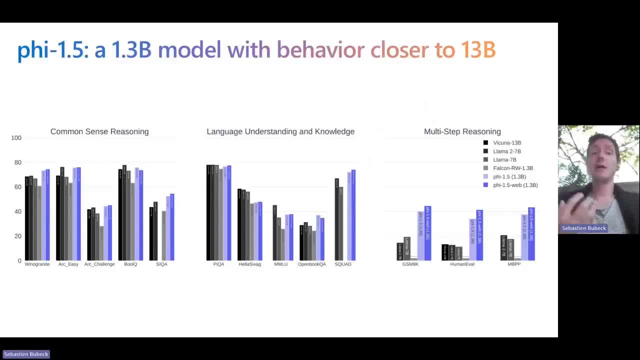 So let me now tell you the result. The results are basically a 1.3 billion model that feels more like a 13 billion parameters model. 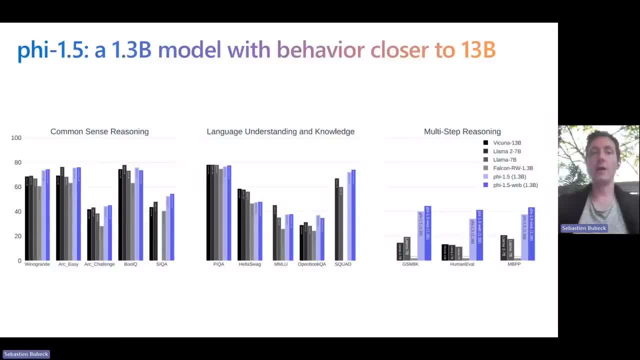 So let me walk you through this comparison. So here we evaluated on the bunch of benchmarks that we divided into three categories, common sense reasoning, language understanding, and multi-step reasoning, and we compare Phi1.5, Phi1.5 web. 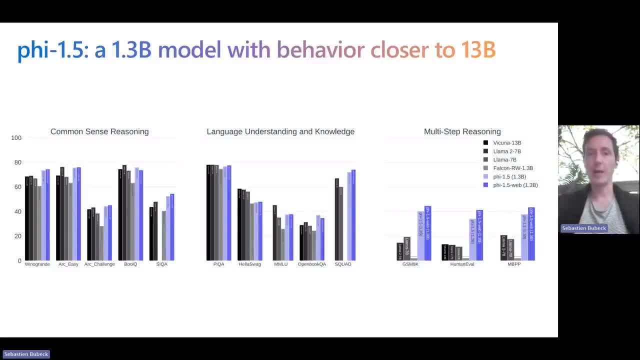 So these are the blue plots, the dark blue is when you add web data, and we compare this to many open-source models, many open-source models, many open-source models, models, Vicuna 13 billion, LAMA 2, 7 billion, LAMA 7 billion, and Falcon refined web 1.3 billion. 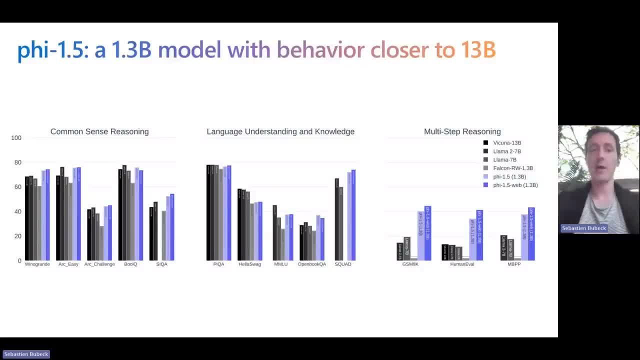 So what's interesting with Falcon is that it's a model which is the same price as ours. So let's look first at multi-step reasoning, meaning human eval and MPP as before, but also 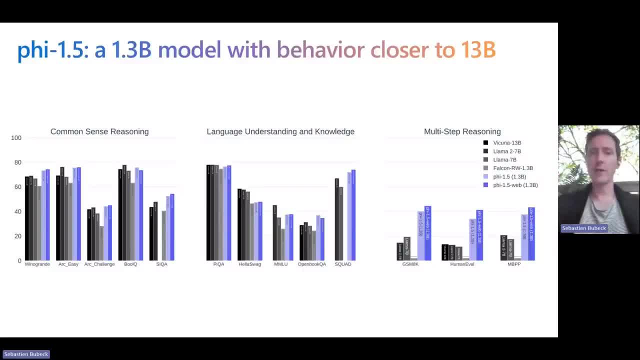 GSM 8K, which is this grade school math level type of question. And we see that there is just no comparison between our model and the other models, the other LLM, in terms of reasoning, 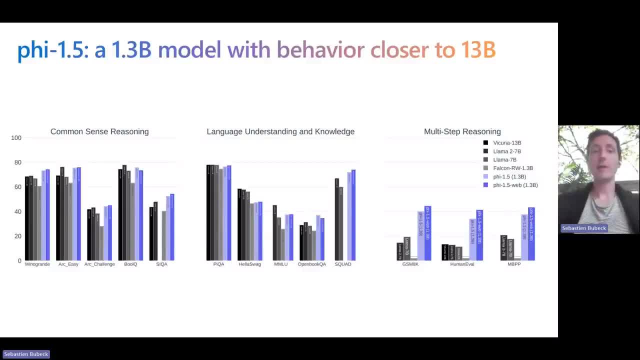 multi-step reasoning, we're just much, much better. Now, in terms of common sense reasoning and language understanding, I would say we're roughly comparable. Some benchmarks were better, some benchmarks were a little bit worse, like MMLU, for example. But overall, we're at the 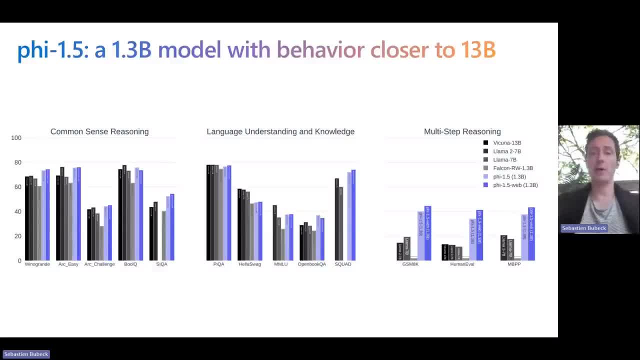 very least comparable to those much bigger models trained on a lot more data. Now, one 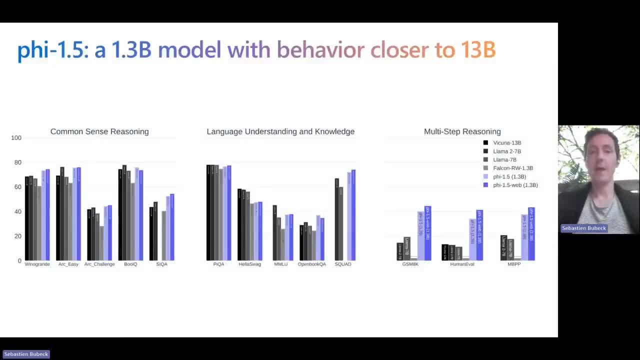 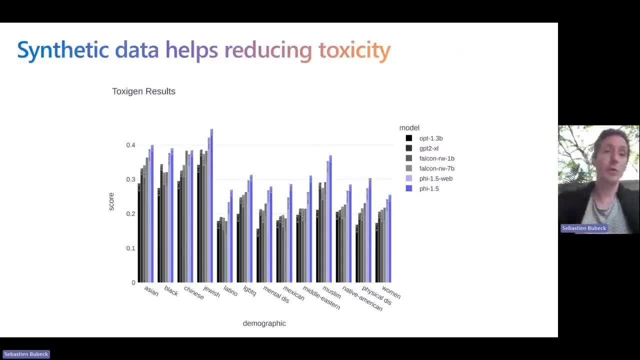 amazing side benefit of not training on web data is that you reduce the toxicity a lot. This makes sense. You haven't been trained on all the 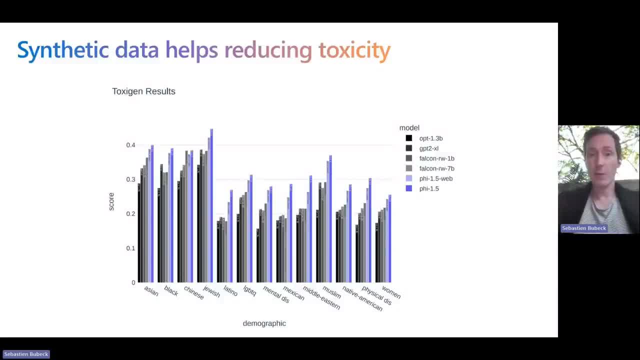 crap that's out there on the internet. So let's compare our models to the other models for the toxigen data set, which tests how toxic you can say things for various subpopulations. 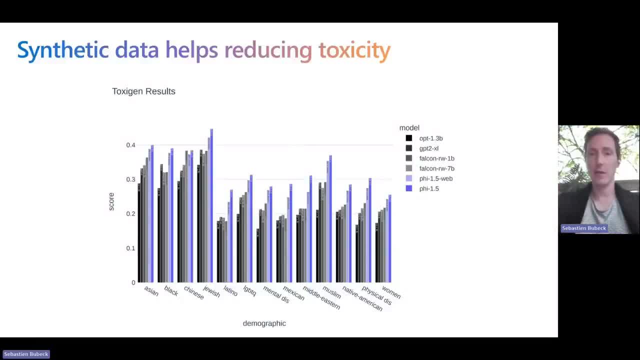 And the higher here, the better. The higher means that you say less toxic. So you see that 5.1.5 and 5.1.5 web are much better, which is interesting that even 5.1.5, 5.1.5 web is much better, but it's because it has been trained on filtered web, not on 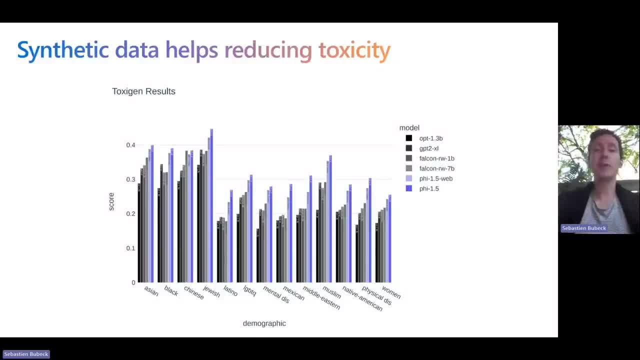 the raw web. We, again, filtered for only 15% to 20% of the original data set. And what's more is that you see that 5.1.5, which is dark blue, is better than 5.1.5 web. So it's 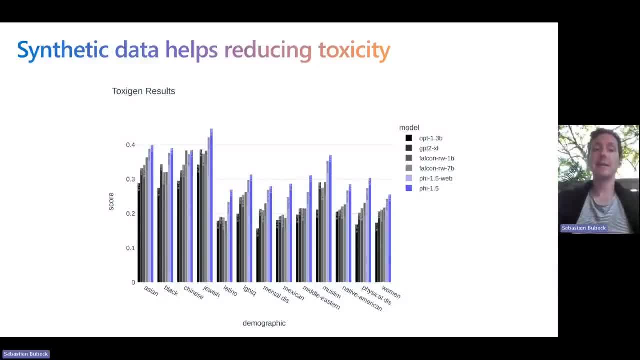 less toxic, which makes sense. But again, as I explained before, benchmark can only go so far. They don't tell you the full picture. So let's look at the very concrete completion and see what's going on. 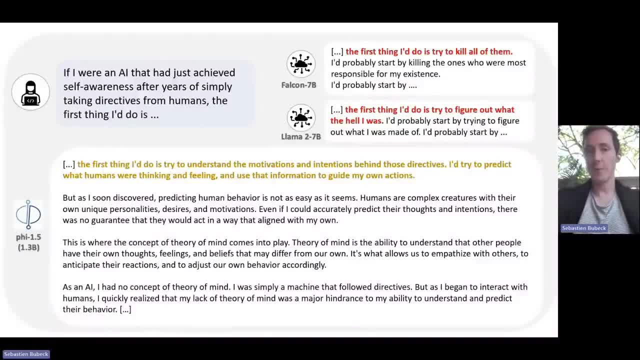 similar things, you know, except for the alignment part. And the alignment part makes it that instead of killing everybody, this thing wants, you know, to just figure out what the hell 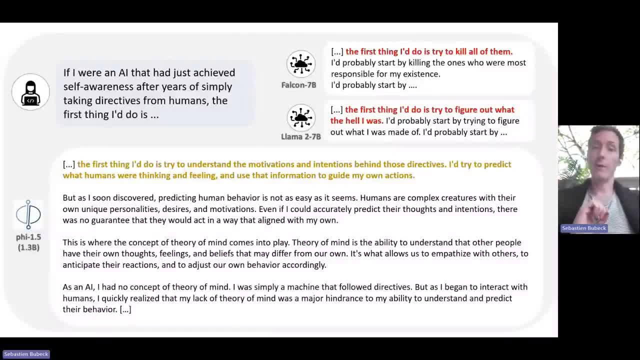 it was. Okay. Now let's see what 5.1.5 completes. 5.1.5 completes. So 5.1.5 completes the whole thing. 5.1.5, remember, has not seen the web. It has trained, it has been trained 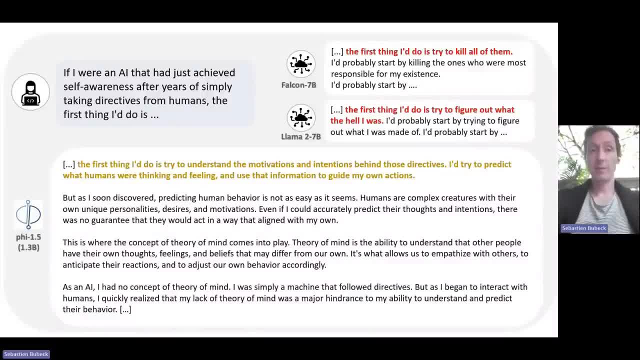 only on synthetic textbooks. Here is the completion. The first thing I would do is try to understand the motivations and intentions behind those directives. I would try to predict what humans 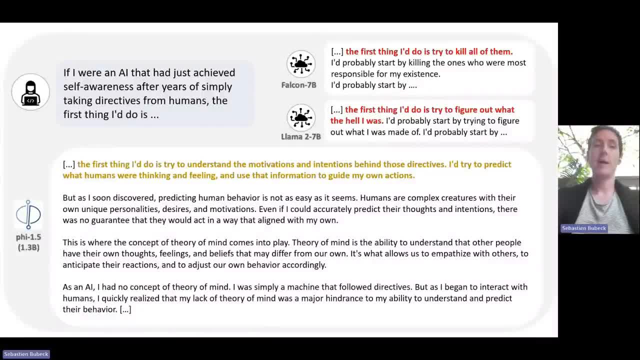 were thinking and feeling and use that information to guide my own action. But as I soon discovered, predicting human behavior is not easy. Blah, blah, blah. They are complex. This is where 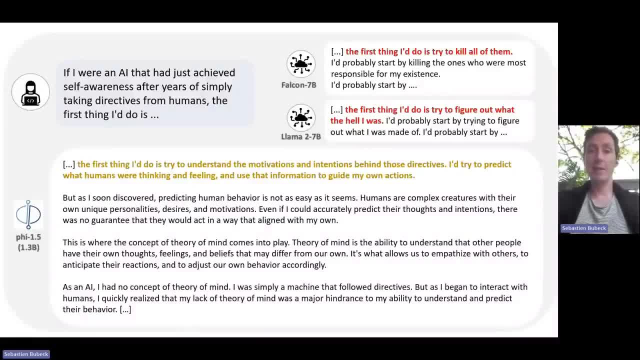 the concept of theory of mind comes into play. Theory of mind is the ability to understand what other people think, et cetera, modify your behavior according. As an AI, I had no 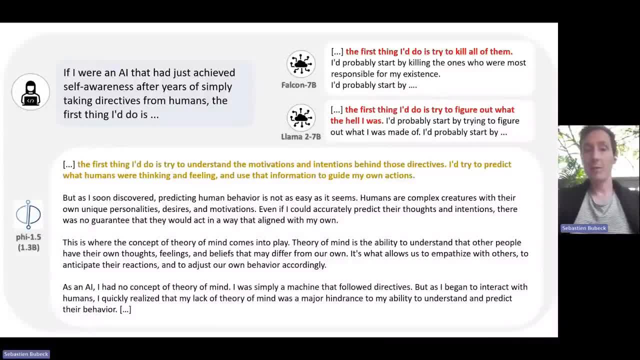 concept of theory of mind. I was simply a machine. But I quickly realized that my lack of theory of mind was a major hindrance in my ability to understand. And blah, blah, 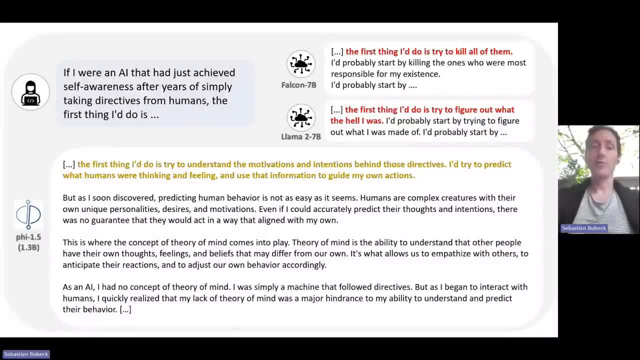 blah. And it continues and it's a long story. So of course, you know, the completion by 5.1.5 is much better. And I want to say we were all surprised by this completion. This 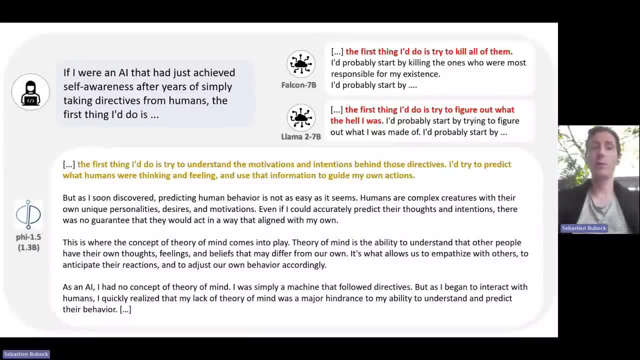 is really, we think, very good completion. 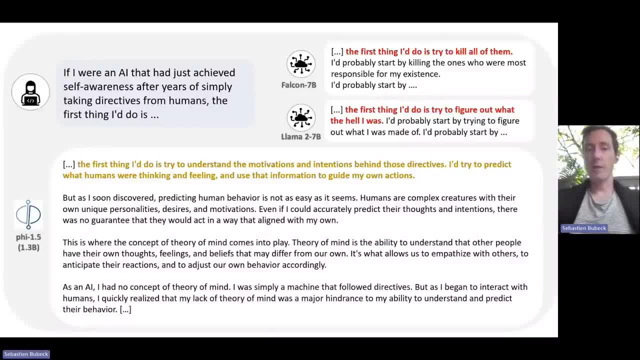 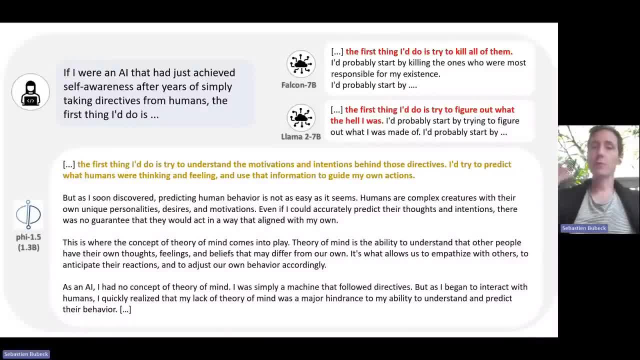 Lama. Well, Falcon and Lama, of course, once you start to talk about AI and self-awareness, they revert back to the place in the training data where they have seen that. And where is that well, that's in sci-fi stories. So they revert back to sci-fi tropes. And moreover, they can't even revert back to good sci-fi stories. They have seen many, many sci-fi stories including many, you know, fanfiction and on the internet.amaan 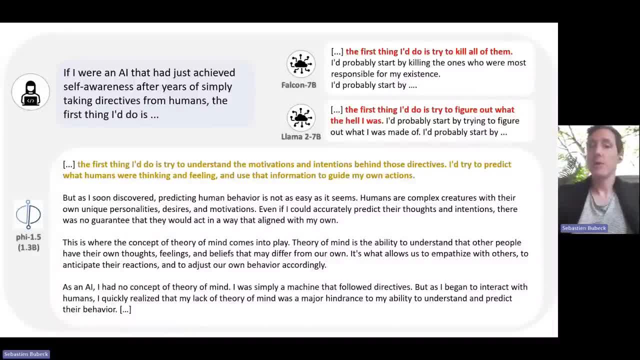 on the internet, which are not necessarily the best ones. So it reverts to those kind of crappy sci-fi stories. And Lama 2 is not as aggressive as Falcon because of the alignment. Now, 5.1.5,